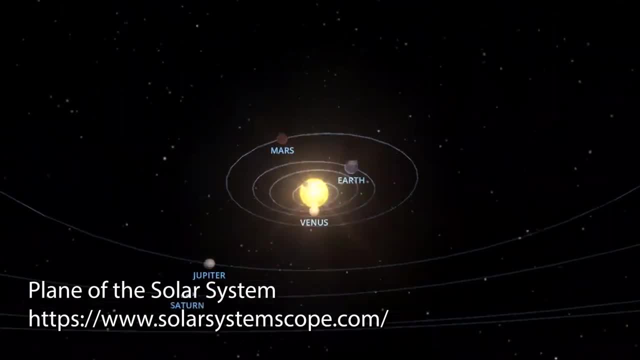 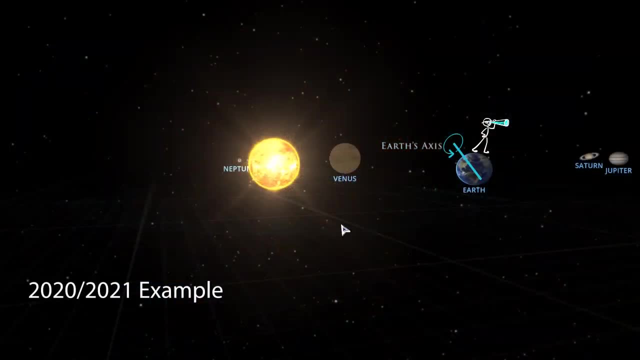 the solar system, And here on Earth we are within that plane. Now here's a fun fact about the ecliptic. Here's me living in the northern hemisphere in the summertime, at night. Here's the sun And here's the ecliptic, or plane of the solar system. Look at where I'm standing on the 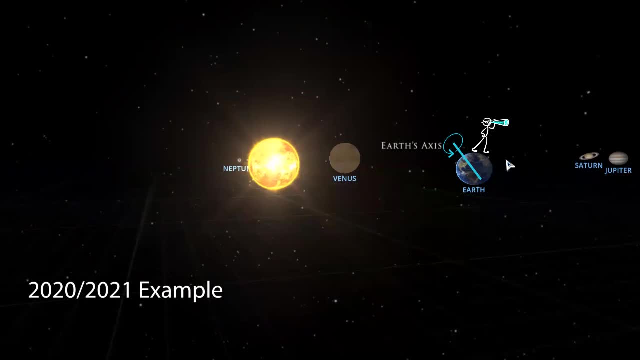 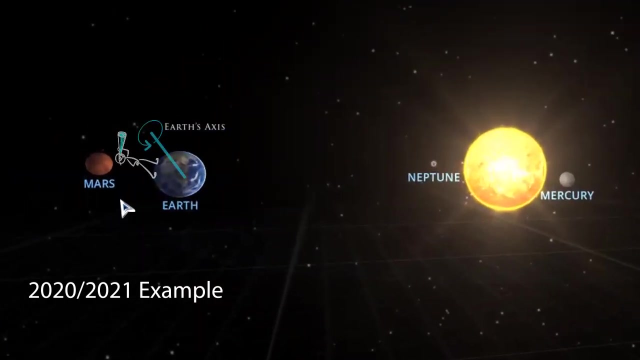 earth, Notice how low the ecliptic must be in the sky. That's why Saturn in 2020, which was in the summertime constellation Sagittarius- appeared so low in the northern hemisphere sky. Now fast forward a few months to winter of 2021.. Here's me living in the northern hemisphere again Now in. 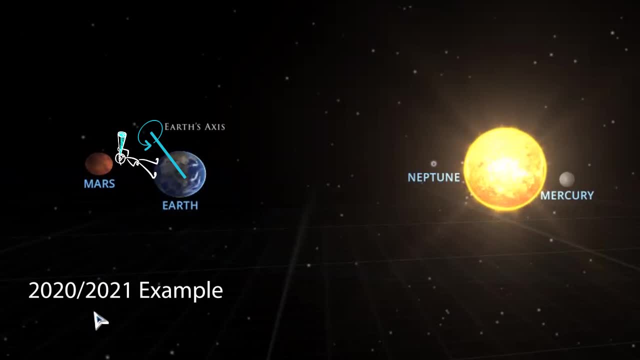 the middle of the night notice how high the ecliptic is. That's why the planet Mars appears almost directly above the ecliptic. That's why the planet Mars appears almost directly above the ecliptic. That's why the planet Mars appears almost directly overhead. So why does this matter? 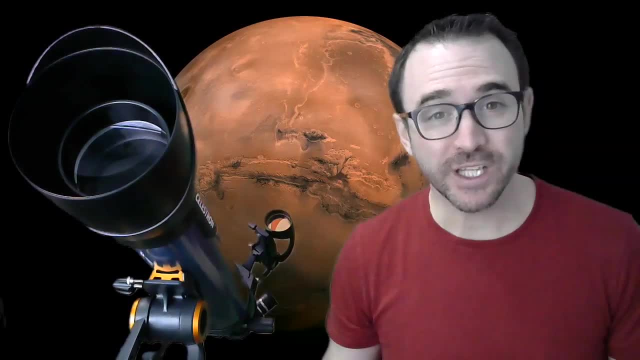 Well, objects overhead offer clearer views because we're looking at them through less of Earth's atmosphere. They're also higher above the horizon and less likely to be blocked by trees or buildings. Venus and Mercury, however, orbit closer to the sun than the Earth and therefore 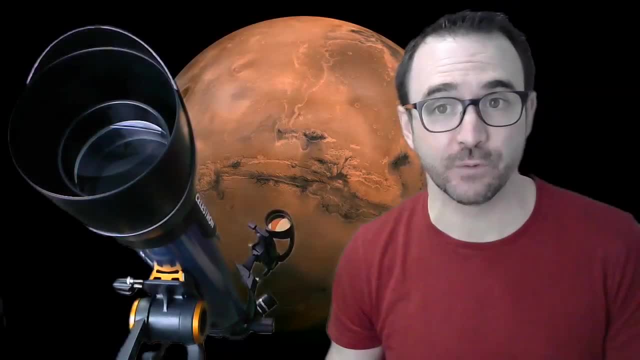 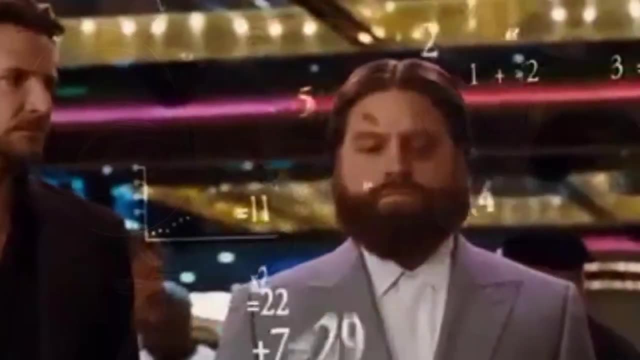 never stray far from the sun and can only be viewed either just before sunrise or just after sunset. And because these are viewed around sunset or sunrise, the ecliptic is highest in the first day for sunset and the first day of autumn for sunrise. And wow, this is getting complicated. 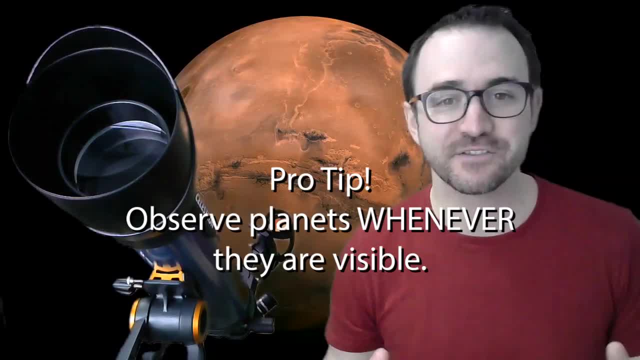 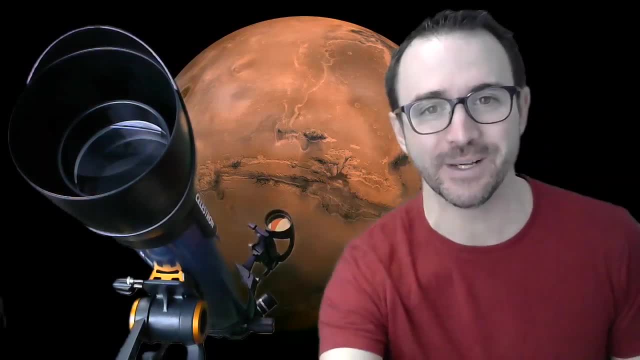 So the best thing to do is not think about anything I just said and try to see planets whenever they are visible, because life is short and if you wait for things to be perfect, you'll probably get clouded out anyway. Now here's an interesting question: Can you see the planets? 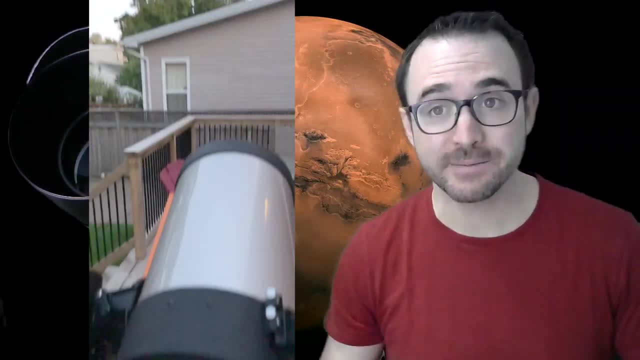 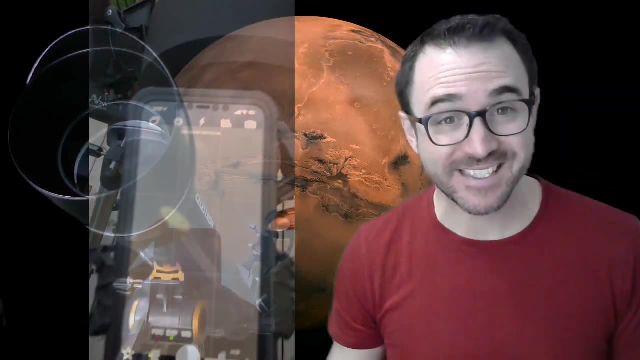 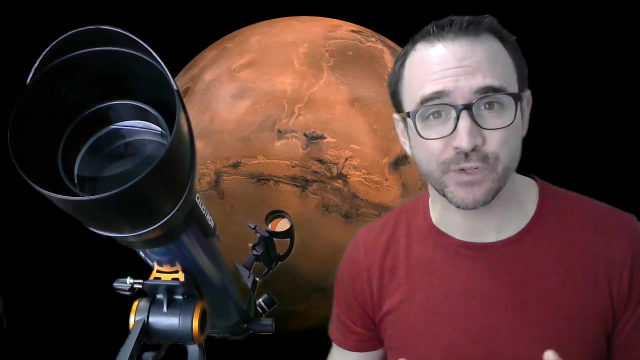 during the day. Yes, with a telescope you absolutely can, though it helps to have a very good computerized telescope, But in fact you can see Venus during the day without a telescope. However, without an object like the moon positioned nearby, it's nearly impossible. for 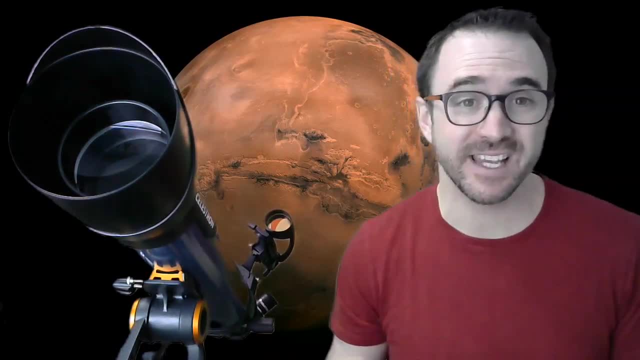 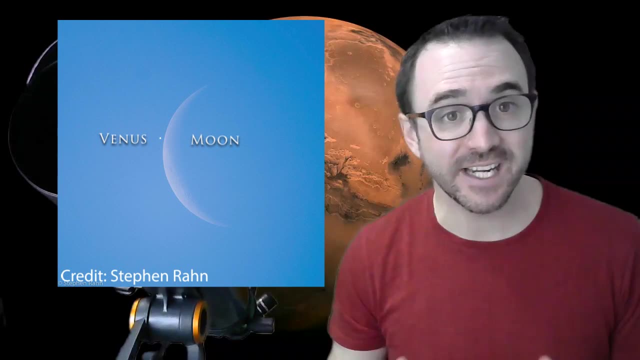 your eyes to focus correctly and all you'll see is blue sky, even if you're looking in the right direction. But if Venus and the moon are very close together, then it's easy to see the tiny white dot that is Venus near the moon. in the daytime sky You can also easily see planets and 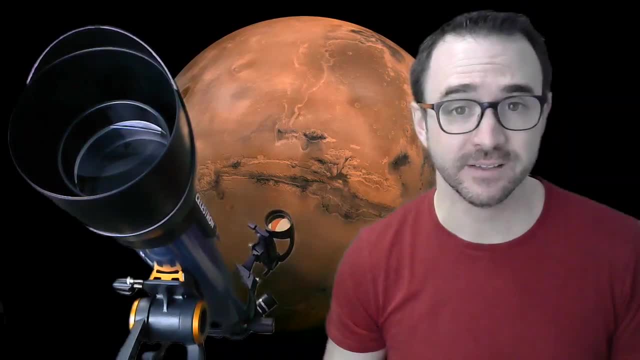 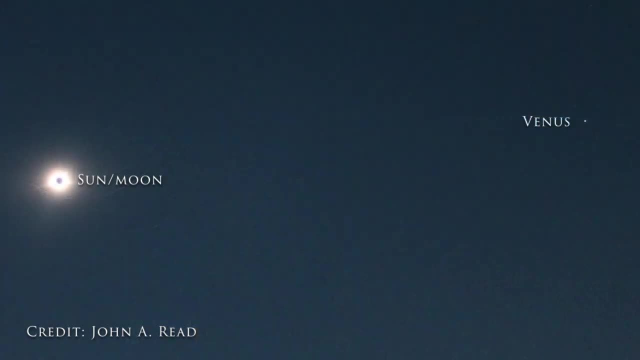 moon in the daytime sky. I was able to see the moon in the daytime sky. I was able to see the moon in the daytime sky. In any case, if you're part of a telescope and you do try to see planets during the day, do NOT point your telescope anywhere near the 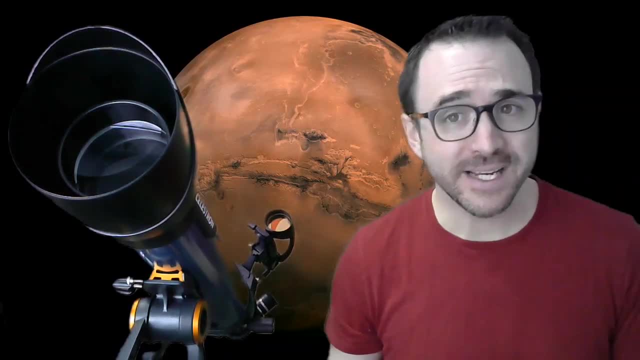 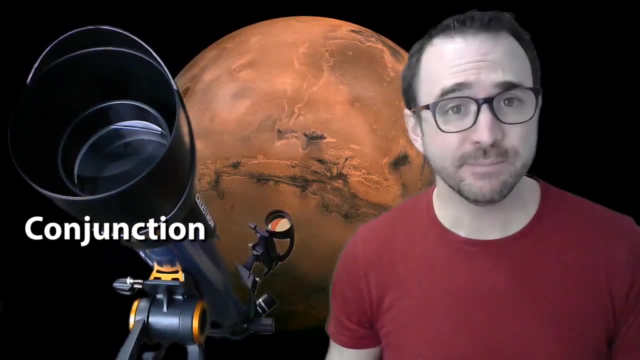 sun… Go blind. Let's get to some terms you might hear when researching the planets. First, you might hear about conjunctions. Well, we talked about conjunctions in a previous video. To put it simply, this generally refers to when two or more planets or the moon appear. 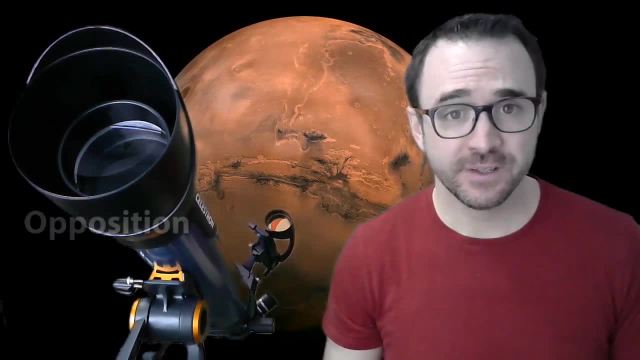 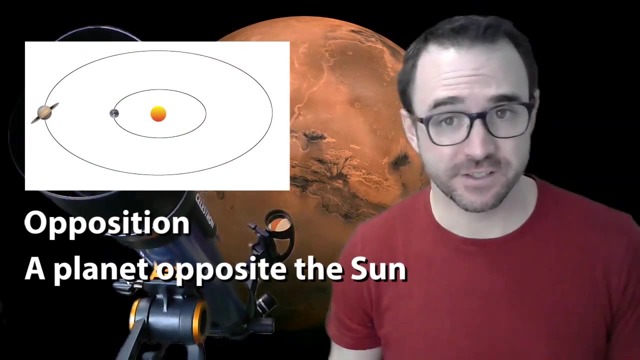 near each other in the sky. You may also hear the term opposition. In addition, this is when a a planet is directly opposite the sun from the earth. this also means that the planet is near its closest to earth and also that it's the highest in the sky in the middle of the night. 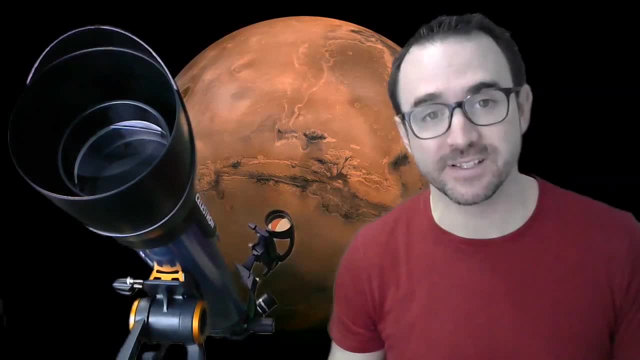 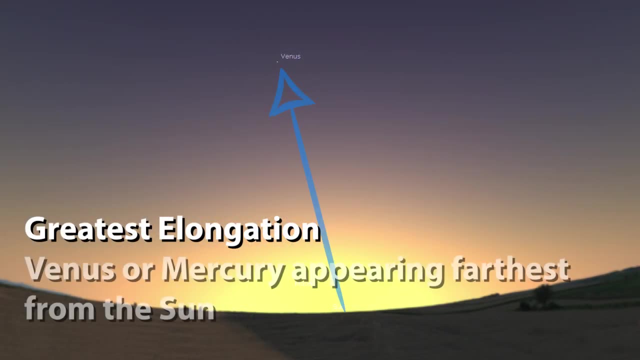 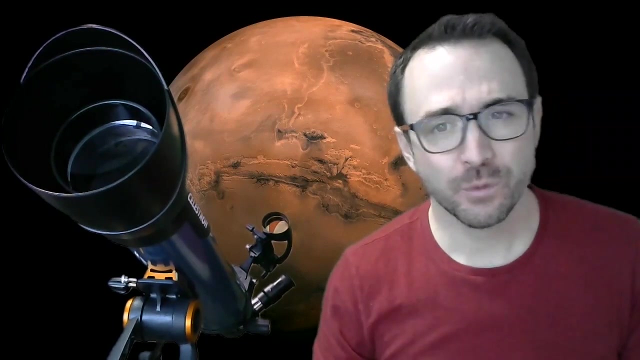 opposition is generally a great time to see a planet with a telescope less frequently. you may hear the term greatest elongation. this only refers to venus and mercury and occurs when the planet appears farthest from the sun when viewed from earth. you may also hear the term retrograde, which 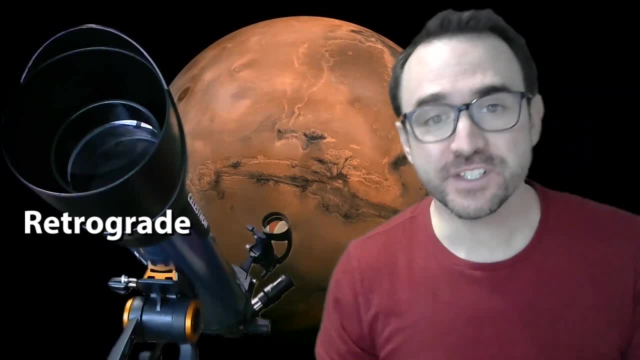 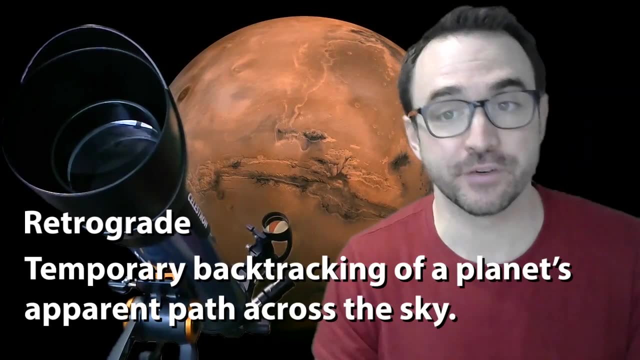 simply means that the earth has passed a planet in its orbit, just like you might pass another car on the freeway. unlike the car you just passed, the planet will briefly appear to be traveling in the other direction as it moves across the sky. to be clear, a planet in retrograde has absolutely no 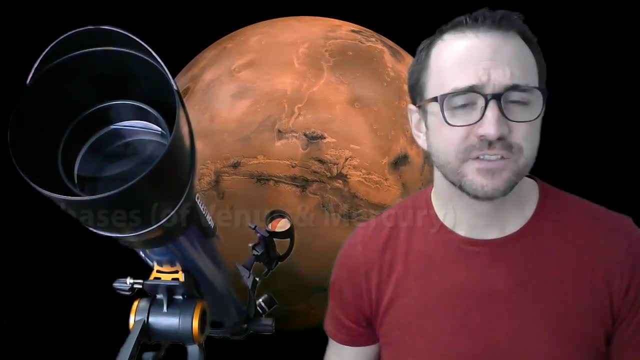 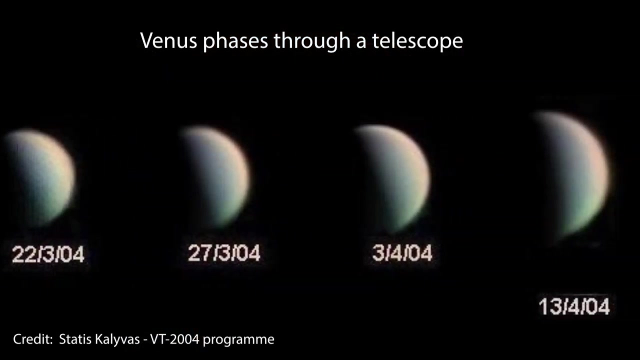 impact on daily life here on earth. and now phases. just like the moon has phases, so do venus and mercury. this is because those planets orbit closer to the sun than the earth and we often face their nighttime signs. these phases may be harder to observe with mercury, because mercury is a challenge to observe. 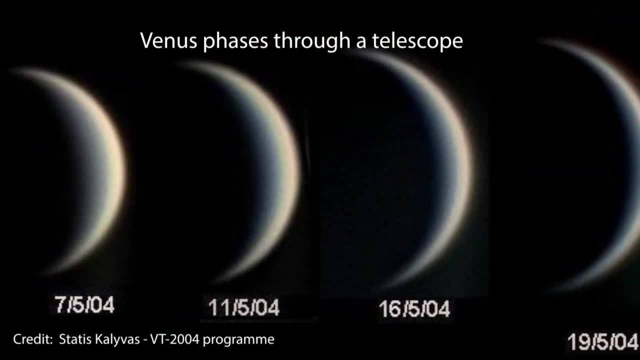 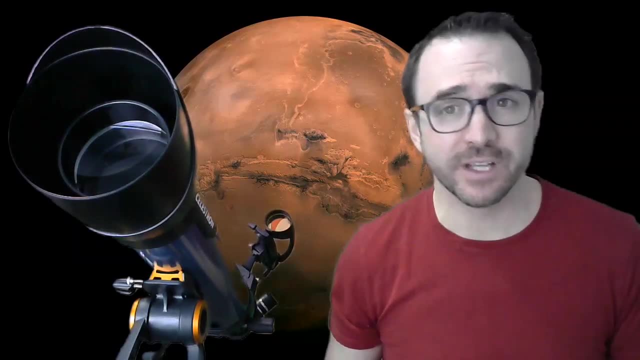 anyway, since it's close to the sun, but with venus, the phases are actually quite pronounced through a telescope. now on to finding the planets. so what's the best way to know what planets are visible on a given night? now there are so many options, all of which work equally well. 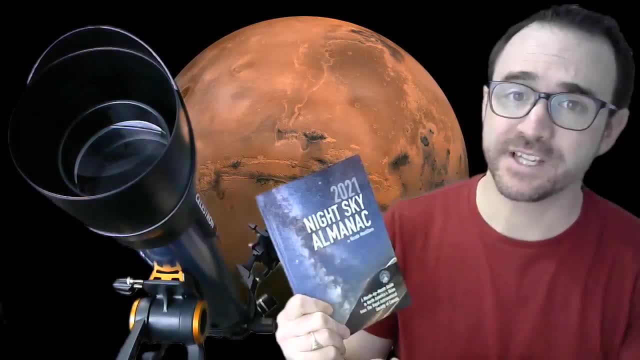 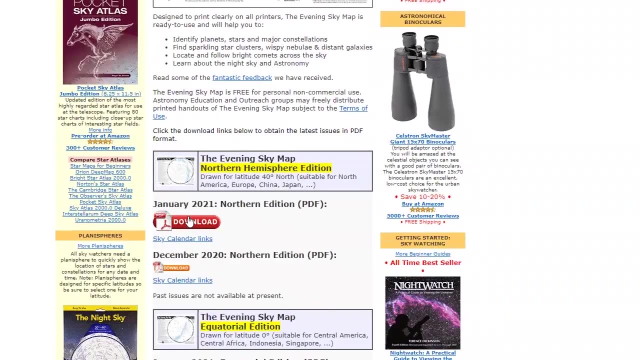 you could subscribe to a magazine like sky news, or you could use the rasc's nighttime almanac for the given year, or you can check the internet. i often use a website called skymapscom and use their evening sky map, but most often what i do is simply check free astronomy. 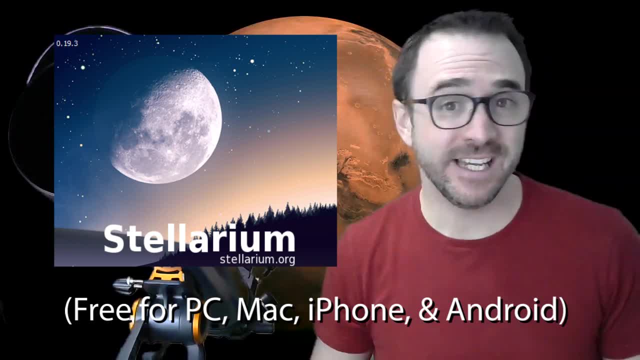 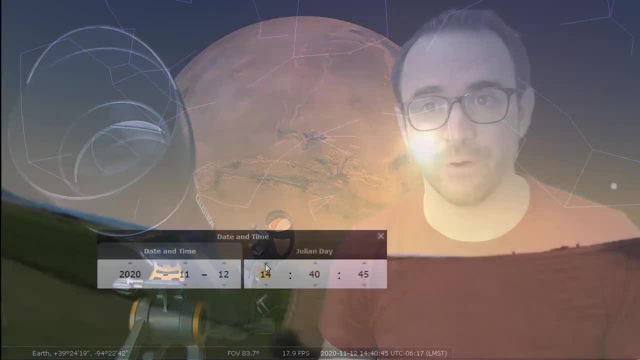 software like stellarium. now i pretty much only stargaze in the evening, within a few hours of sunset. so when i use stellarium to learn what's up, i just set the time to approximately an hour after sunset and then fast forward a few weeks to see what the planets are doing. be sure to select. 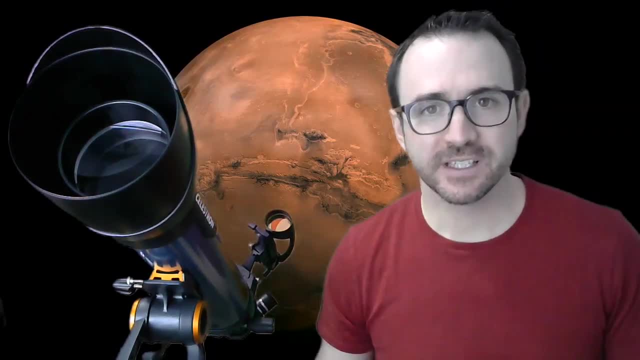 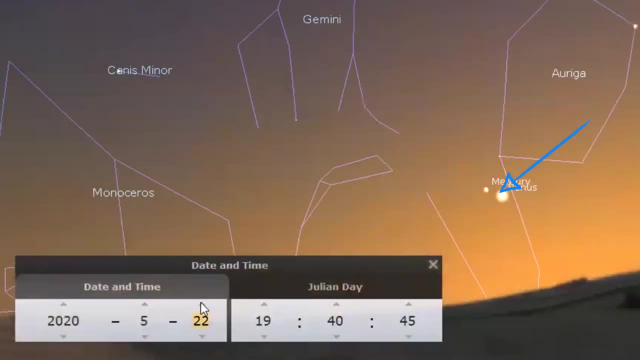 planets from the bottom menu. so, as an example, let's look at the spring, summer and fall of 2020- 2020.. We started the year with Venus high in the sky. after sunset, Mercury makes a brief appearance, then we have Saturn and Jupiter hanging out over here in Sagittarius, Mars. 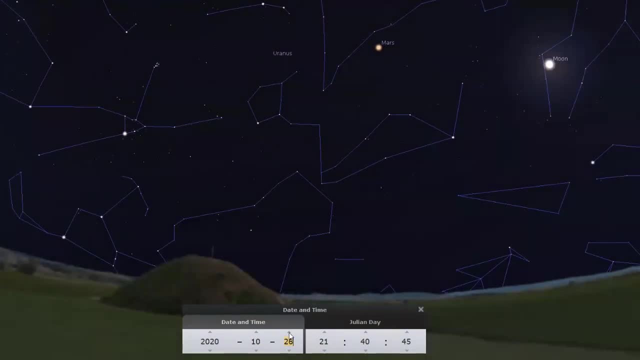 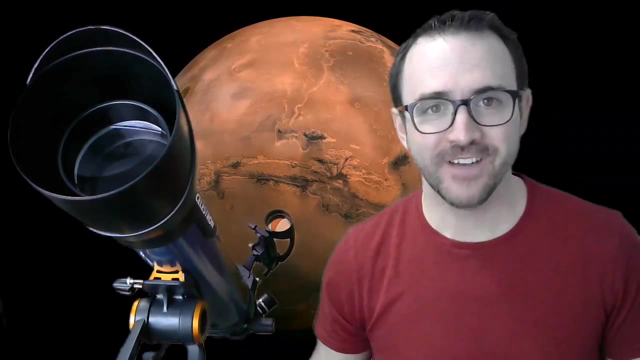 is high in the sky as it reaches opposition, providing incredible views even through small telescopes. We end 2020 with a beautiful conjunction of Jupiter and Saturn. And finally, how do we find these planets in our telescopes? So, from this point onward, 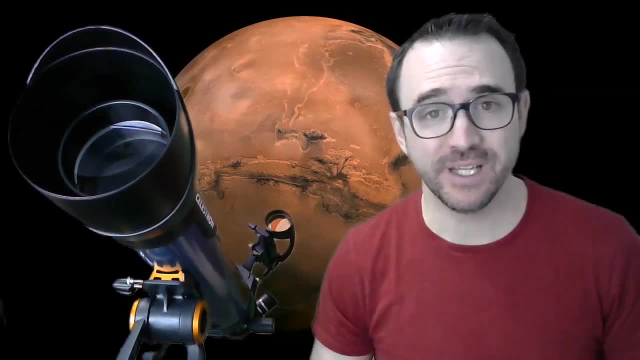 I'm going to assume that you've determined exactly where the planets are going to be on the night that you're doing your observing. This is January of 2021, so I'm going to use Mars as a quick example. You can see it here, to the west of the constellation Orion. 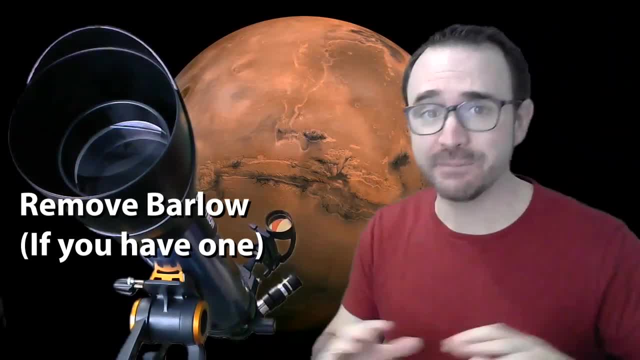 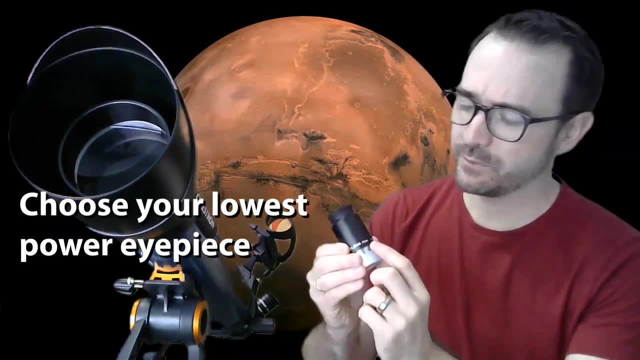 When first attempting to view a planet, make sure you remove any barlows from your telescope. Choose your lowest powered eyepiece, That's, the one with the highest focal length. The focal length of the eyepiece is always written right on. 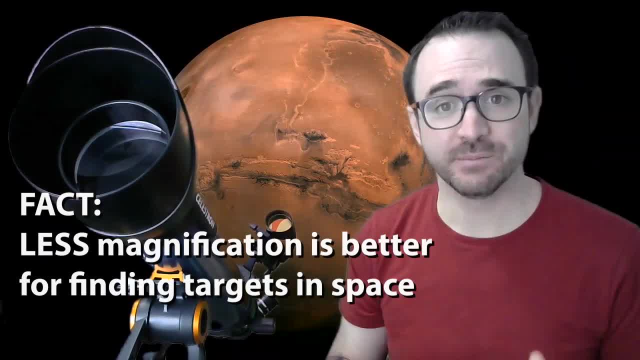 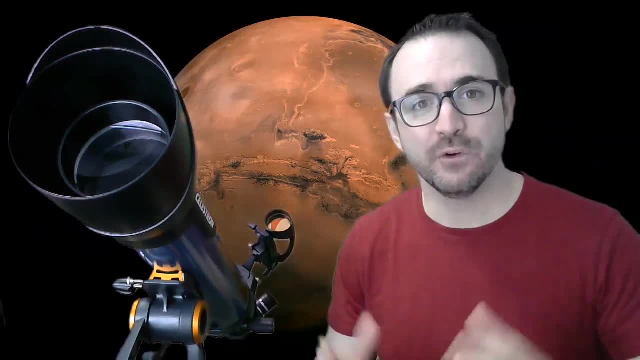 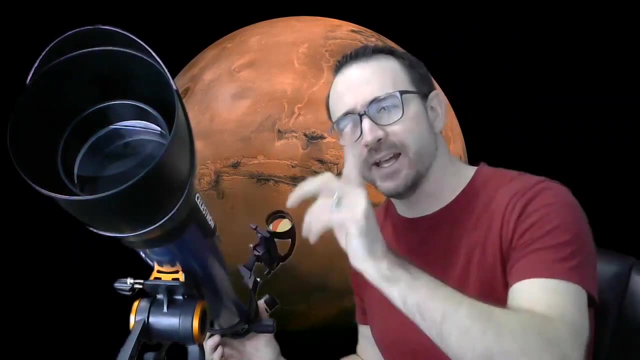 Using as little magnification as possible will make the planet much easier to find in the telescope. So now that you can clearly see the planet in the sky without the telescope, now you take your telescope and point it in the general direction of the planet. Then 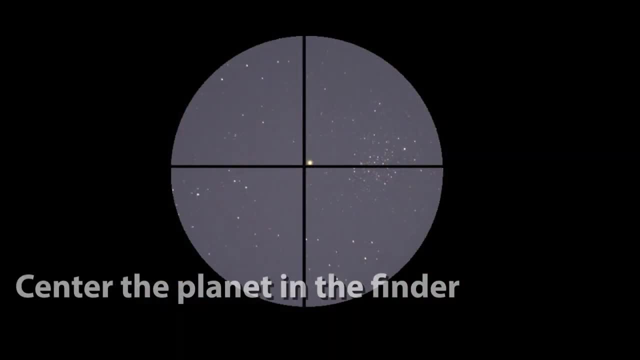 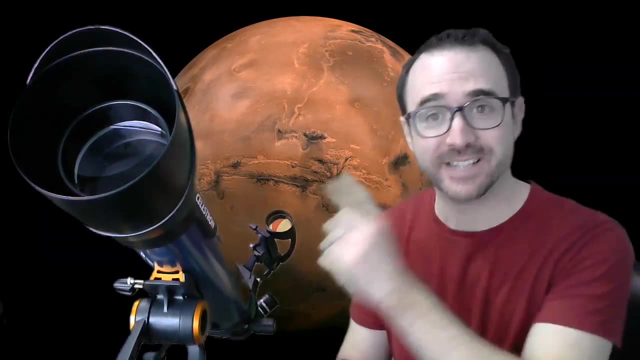 you move to your finder Center- the planet precisely in the finder- and then move to the eyepiece. If the planet does not appear in your eyepiece, then the telescope and the finder are pointed in different directions and you'll want to go back to video number 22 in this series. 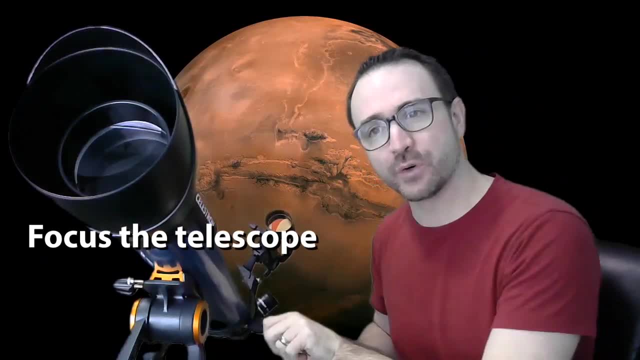 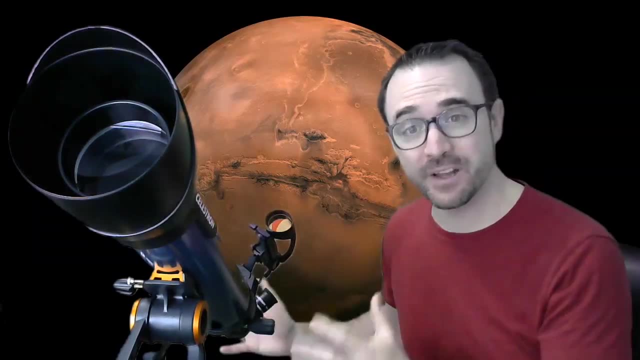 How to Use a Beginner Telescope. Now take the time to make sure that your focus is perfect, remembering that the focus may be unique to your prescription. So if you're stargazing with others, make sure you teach them to focus the telescope for themselves. Planets should appear as crisp. 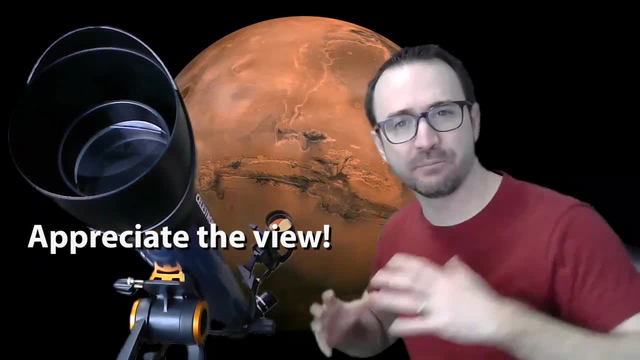 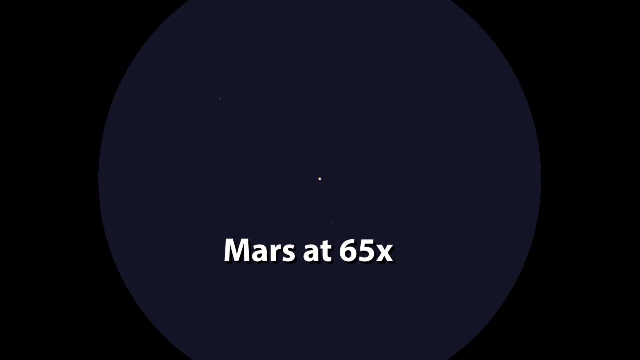 and clear as possible. Now take a moment to observe and appreciate the planet at this minimal magnification. If it's much, then you can just move the telescope to the other side of the telescope. If it's Mars, it'll probably look like a bright red star, but if it's Jupiter, you'll see. 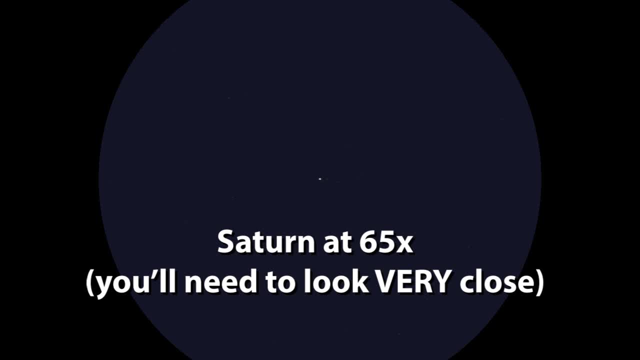 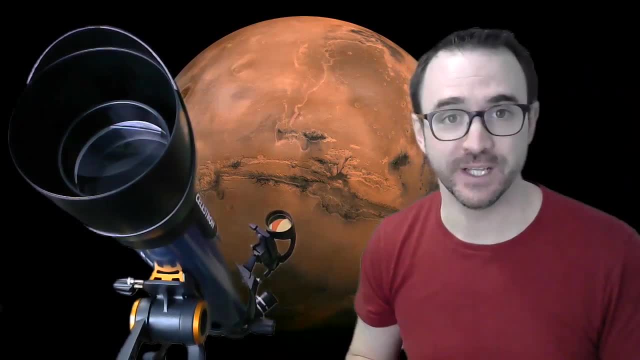 the four Galilean moons, and if it's Saturn, though small, you should still be able to see the rings. Once you've mastered observing the planets at low magnification, now it's time to zoom in. You do this by removing the low-powered eyepiece. In my case, this is a 20-millimeter. 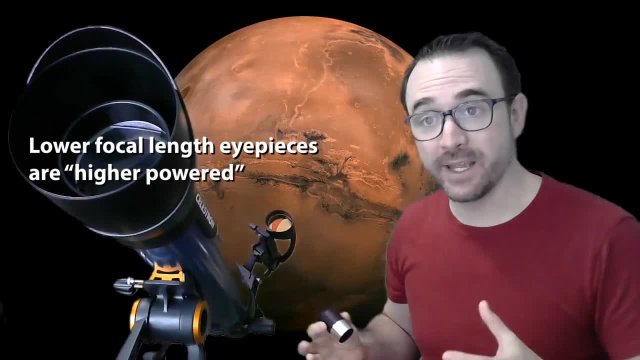 eyepiece and adding a higher-powered eyepiece. In my case, it might be the 10-millimeter eyepiece that came with this telescope. Now look at the telescope. If it's Jupiter, you'll see the four Galilean moons, and if it's Saturn, 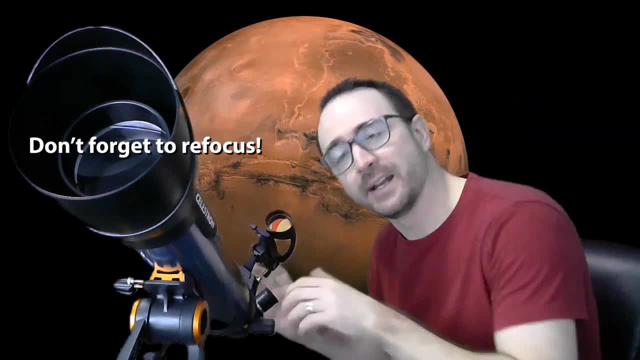 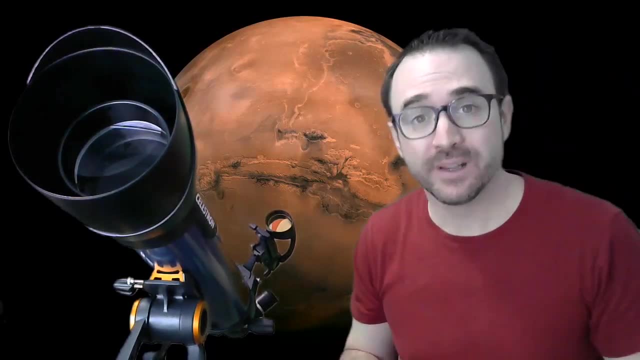 you'll still be able to see the rings Once you've mastered observing the planets at low magnification. now look through the eyepiece again, center the planet and again refocus until the planet is clear and crisp, And finally to zoom in even more. now we add the Barlow, Remove the eyepiece. 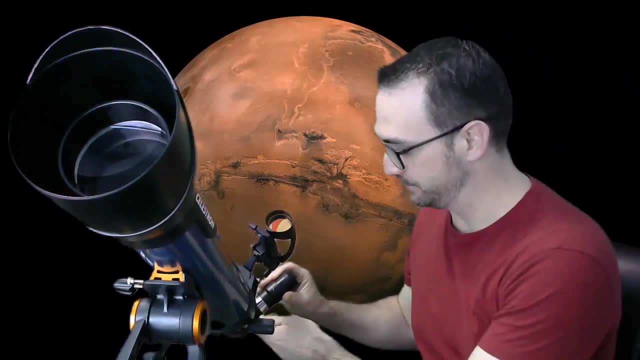 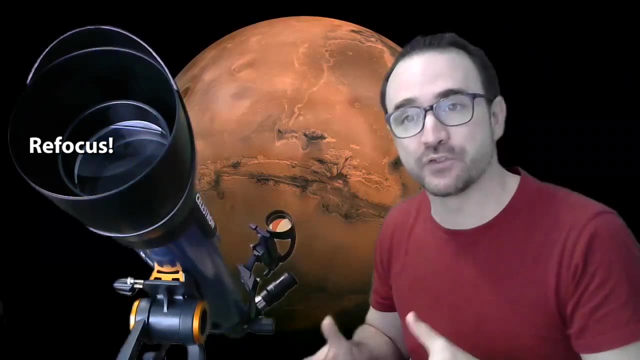 and put the Barlow between the eyepiece and the telescope And again you'll need to look in the eyepiece, center the telescope and refocus the telescope, making sure the planet is clear and crisp. If you've lost the planet, you may need to remove. 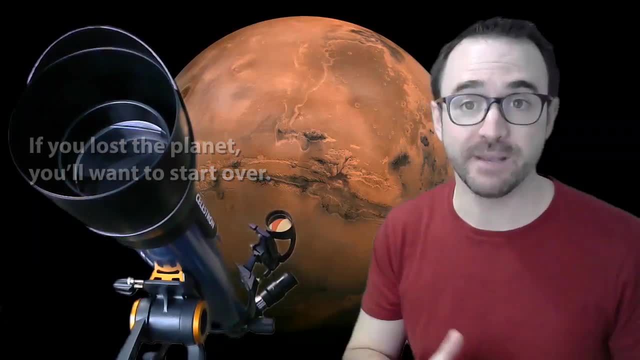 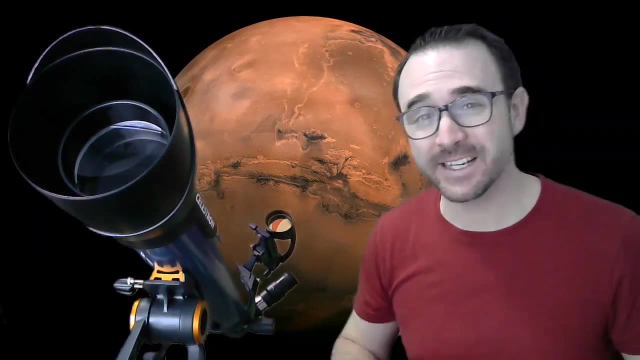 the Barlow and return again to the lowest-powered eyepiece, starting the process over. You may also notice that although the Barlow allowed you to zoom in, it didn't necessarily improve your view. This is because you may be approaching your telescope's. 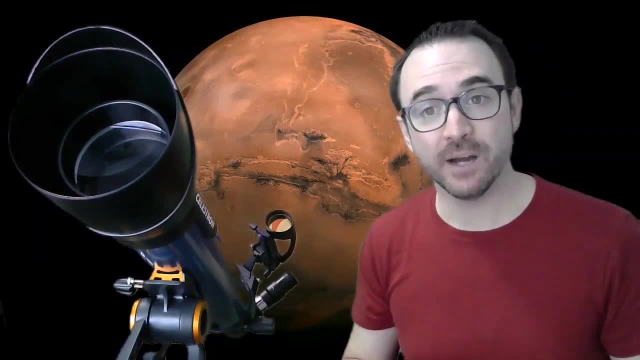 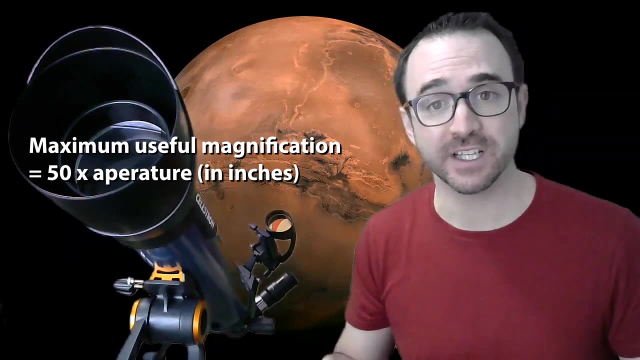 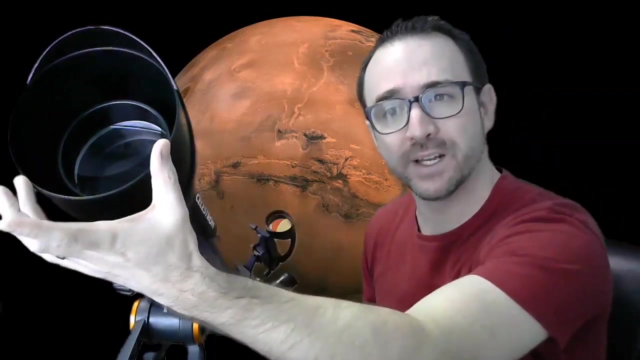 maximum useful magnification, in which case the objects will appear slightly blurry, no matter how much you try to focus. To determine the maximum useful magnification of your telescope, take the aperture in inches and multiply it by 50.. This telescope has an aperture of about 4 inches and therefore has a maximum useful magnification. 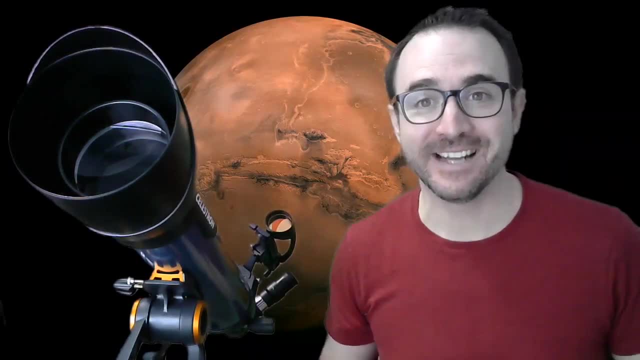 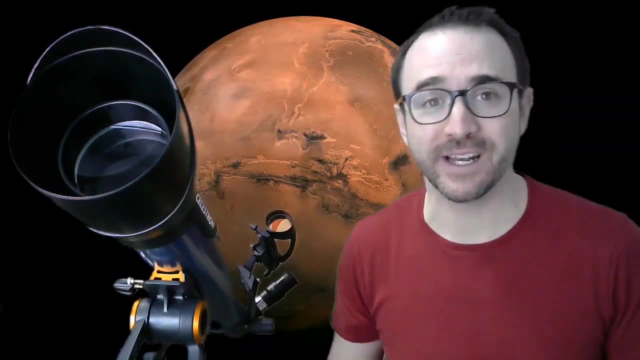 of about 200.. Now, before we talk about Uranus and Neptune, I have a quick message for beginner telescope users. Telescopes can be frustrating. Maybe you're having trouble getting the scope set up and focused and maybe you're having trouble finding cool stuff to see in the sky. 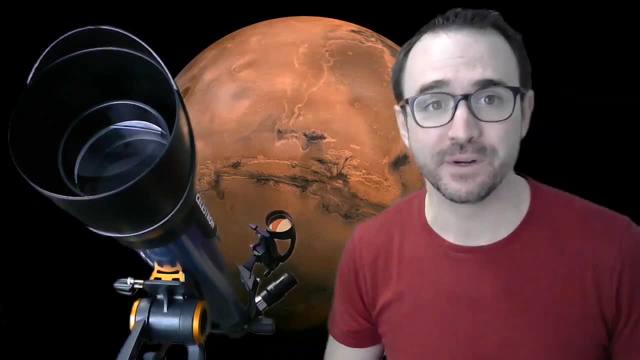 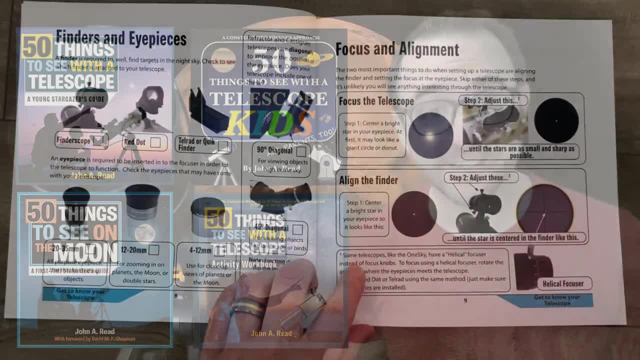 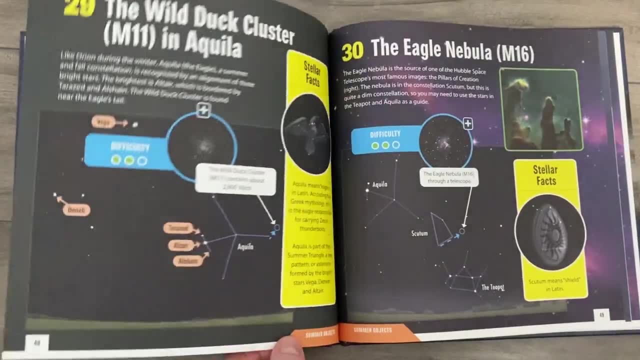 telescope series. This series solves the 50 things to see with a telescope series. This series solves these problems. Each book starts with clear instructions on how to use your telescope and then shows you how to find cool stuff in the night sky. Most importantly, it shows you exactly. 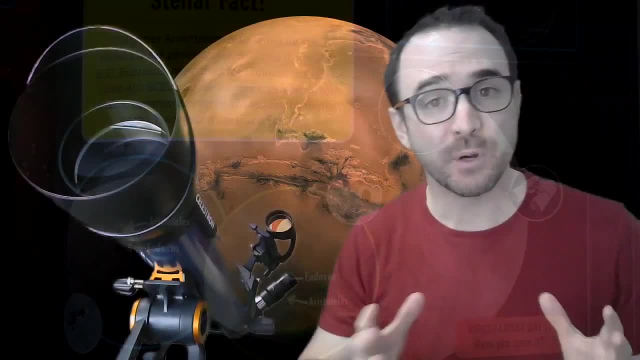 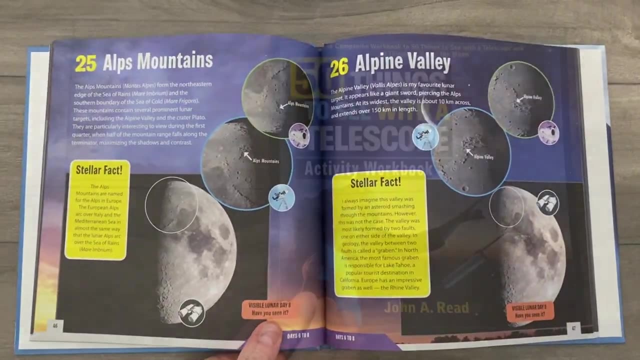 what you should expect to see through your eyepiece. From our most popular book 50 Things to See with a Telescope, to the award-winning 50 Things to See on the Moon and the teacher-friendly 50 Things to See with a Telescope Activity Workbook, there's something for you If you enjoy. 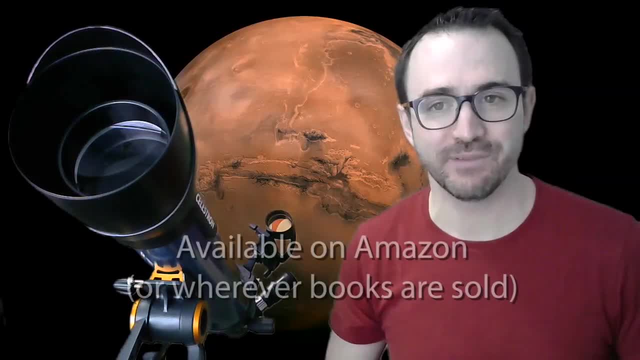 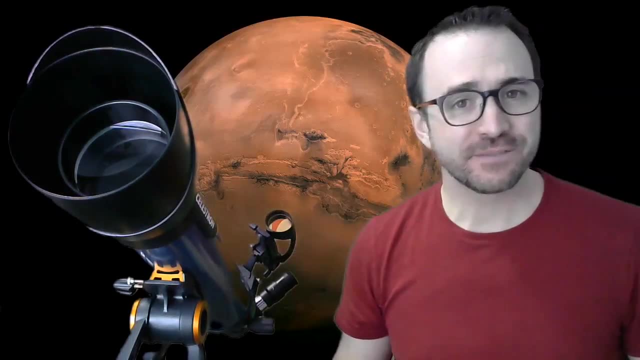 the content here on Learn to Stargaze. please consider one of these books. I guarantee it will vastly improve your stargazing experience. Now back to the planets. So so far in this video we've looked at how to find planets that are visible to the naked eye. But what about Uranus? 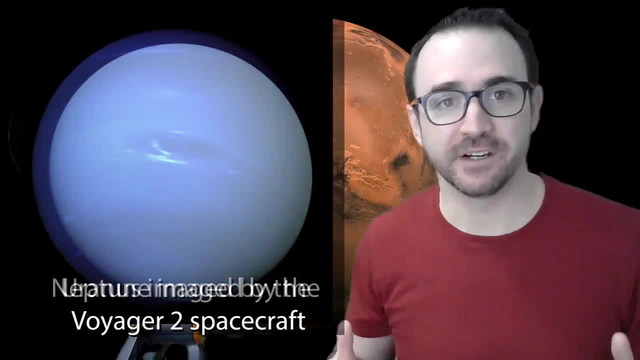 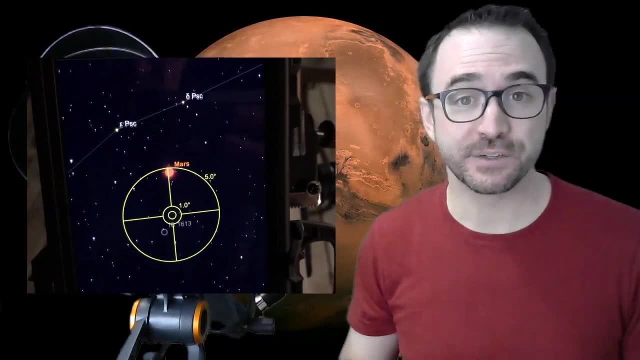 and Neptune. These planets can be challenging to find in backyard telescopes. They are easiest to find with a computerized telescope or with the new Celestron StarSense which uses your phone to precisely point the telescope. But if you don't have a telescope, you can use a telescope. 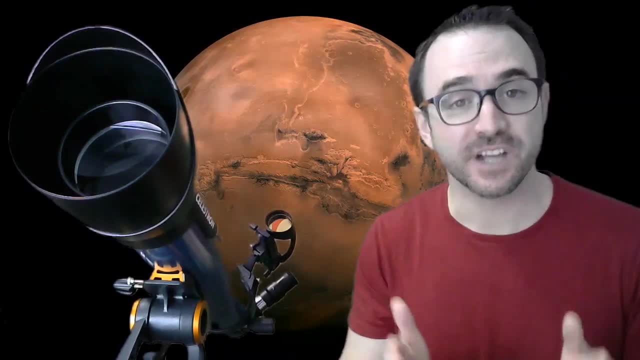 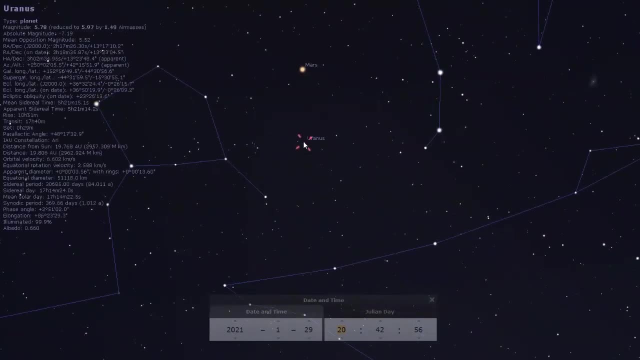 If you have any type of computerized assistance, you'll have to star hop to the planet. To do this, bring up the planet in astronomy software and note exactly where it is, using neighboring stars as a reference. Build a set of directions to the planet based on these reference stars. 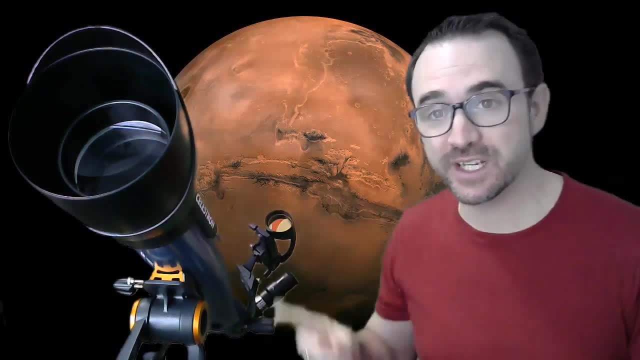 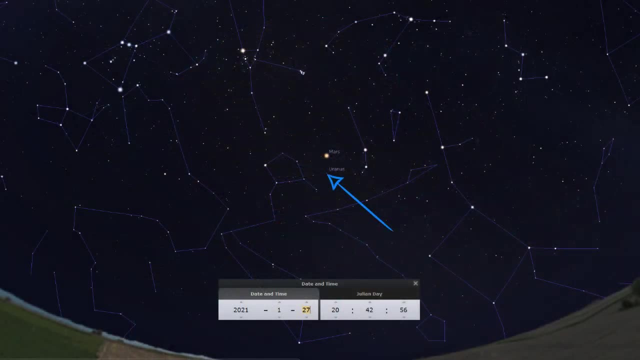 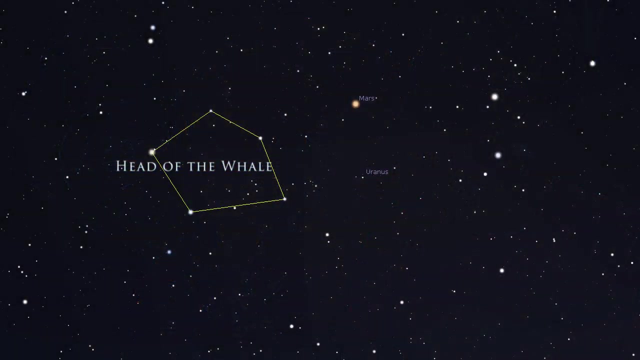 and point your telescope precisely at this location using your finder As an example. here's Uranus as it appears tonight, January 27, 2021.. Here we can see that Uranus is located near Mars and near this hexagon of stars which is an asterism called the head of the whale. Using Mars. 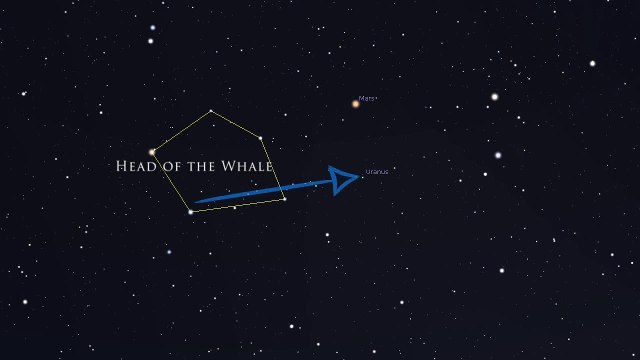 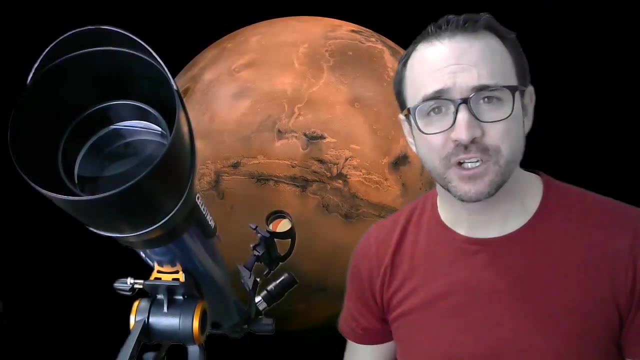 and the base of this asterism. we can star hop to Uranus by forming a right angle, as shown Now. we just point the telescope exactly at this spot And if you're using a finder scope, you may be able to see Uranus or Neptune in the finder as a small bright dot, assuming the finder. 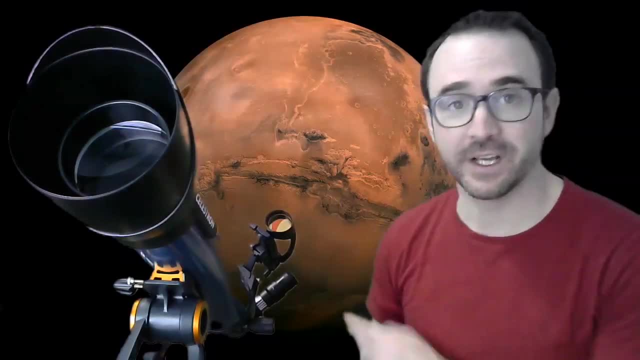 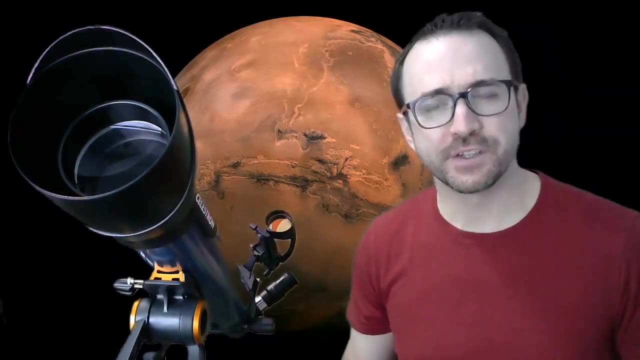 scope itself is powerful enough. If you're using a red dot finder or a Taurad like this one, you won't see it, since these finders do not provide any magnification. Even if you're searching for Uranus and Neptune, you'll want to start with the lowest powered eyepiece As soon as you've found. 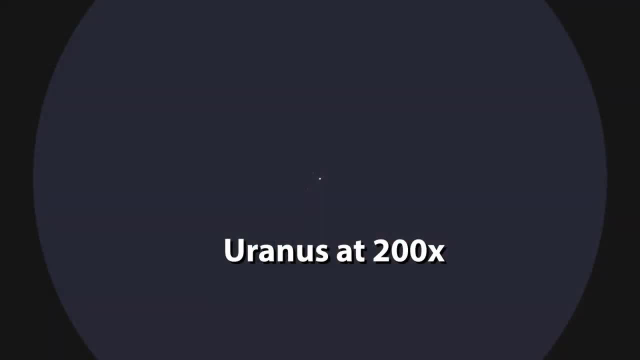 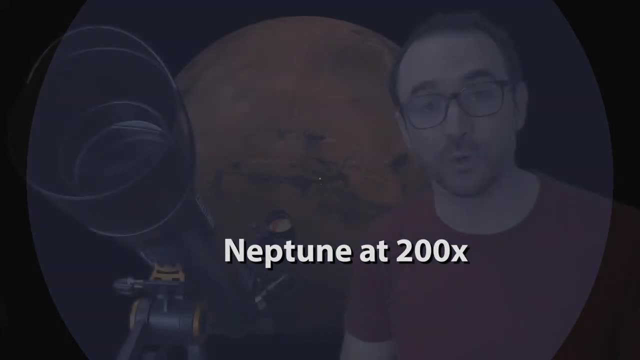 it, then you'll want to move up to higher powered eyepieces and maybe even the Barlow. Depending on the size of your telescope, you may be able to resolve the planet's disk and see one or more of its moons Moving on. now I've been getting a lot of questions about zoom eyepieces for viewing. 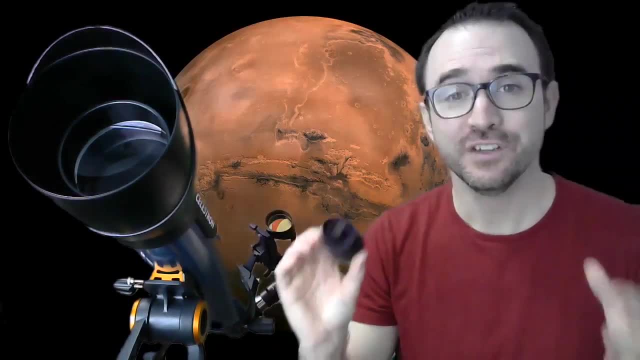 planets like the Celestron 8-24mm. Should you get the Celestron 8-24mm eyepiece or should you get the Celestron 8-24mm eyepiece? or should you get the Celestron 8-24mm eyepiece or should you get? 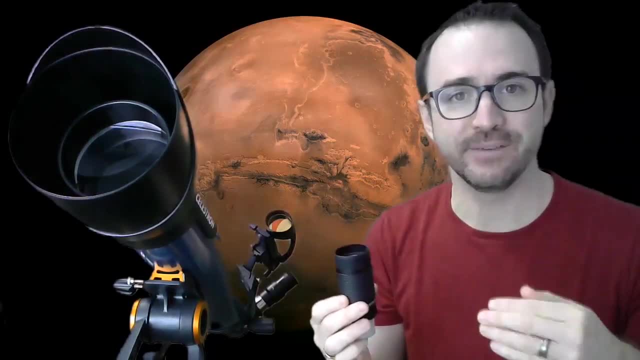 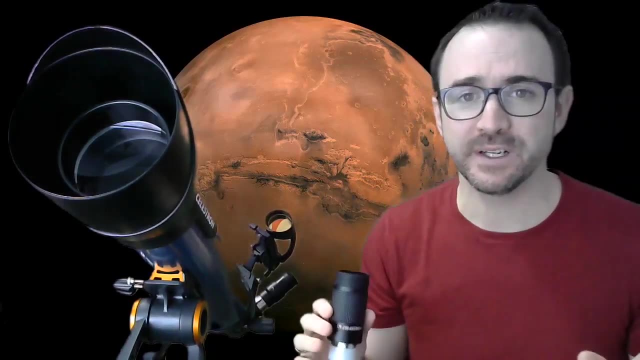 one. Well, a zoom eyepiece simply saves you from having to switch eyepieces to zoom in, So if you think that's worth the cost, then go for it, But it's not a whole lot different than just using the two eyepieces that probably came with your telescope. Well, after you've found a planet that? 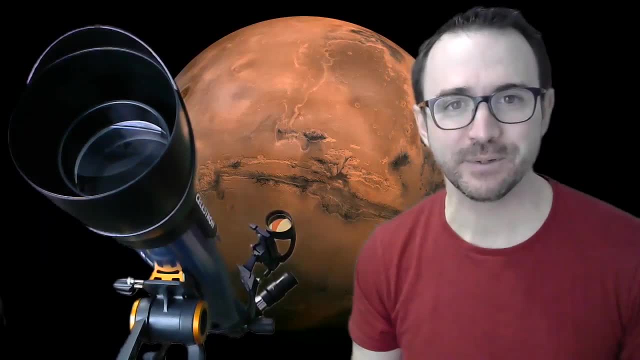 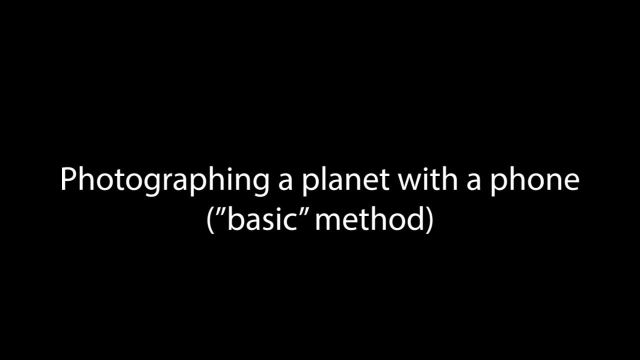 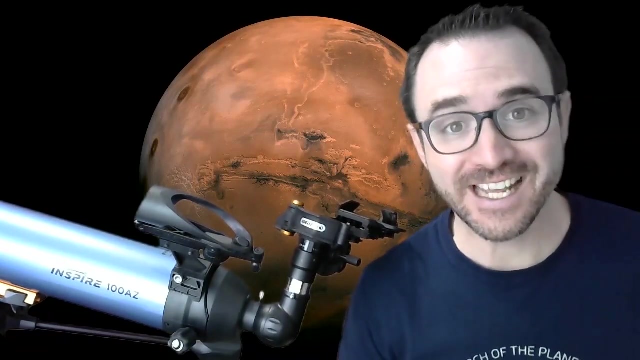 looks cool to your eye, like Saturn, and if you're like most people, you'll want to photograph it and share that photo with your friends. So here's how you do that. So when taking a photo of a planet with a cell phone, there are a few things you'll want to consider. First, it takes practice and a lot. 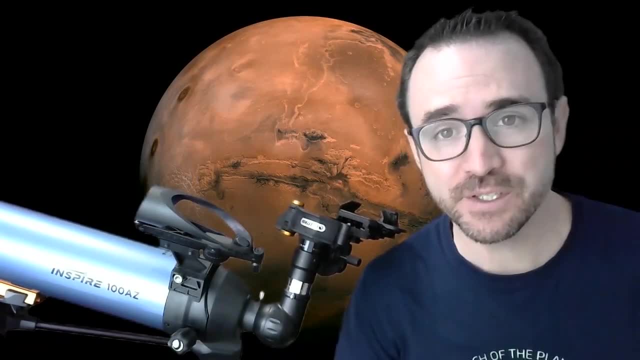 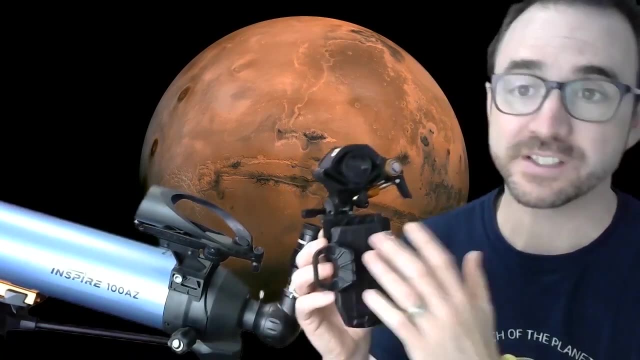 of practice, The phone must be lined up perfectly for the image to appear on the screen. That's why it helps to have a phone adapter like this one. And for those that are wondering, this is probably the best cell phone adapter there is. This is the Celestron NextYZ. Now I'm going to show you what. 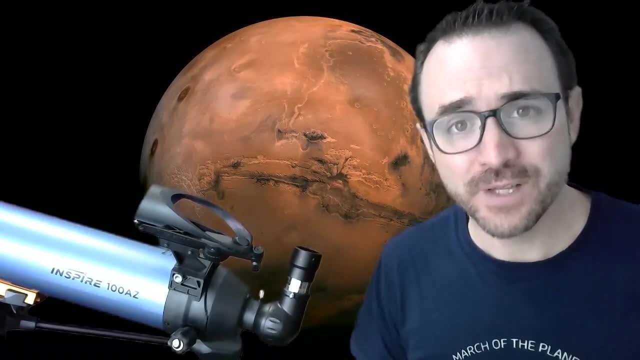 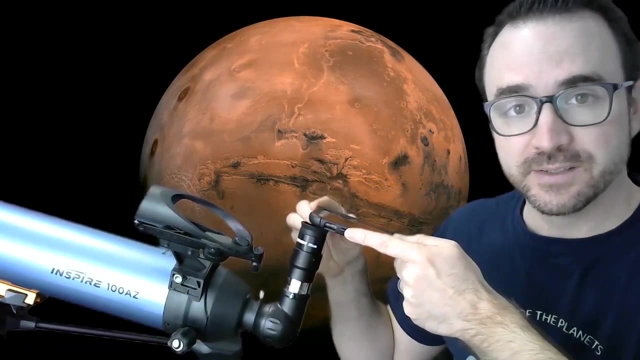 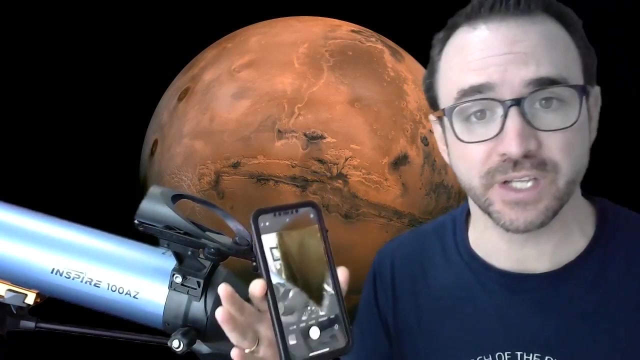 it looks like to do this without the phone adapter. For this video, we're just going to use the eyepiece and hold the phone up to the eyepiece to take the picture. The second thing you'll want to consider is the camera app you're using to take the picture. Now, I usually use the standard app that comes with. 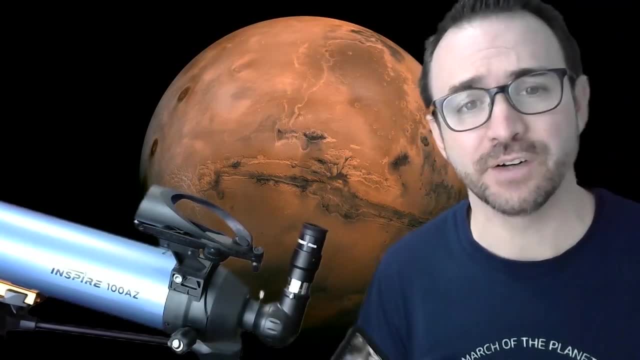 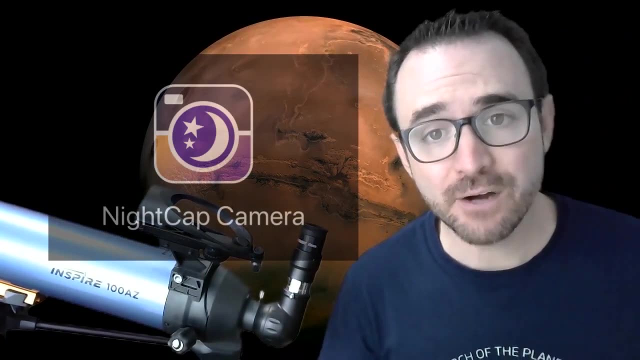 the camera, but the challenge here can be getting focus and setting the correct exposure. It's important that the planet not be too bright or overexposed. Using an app like Nightcap allows you to lock the focus and the exposure, because you need the planet to appear decently on the screen. 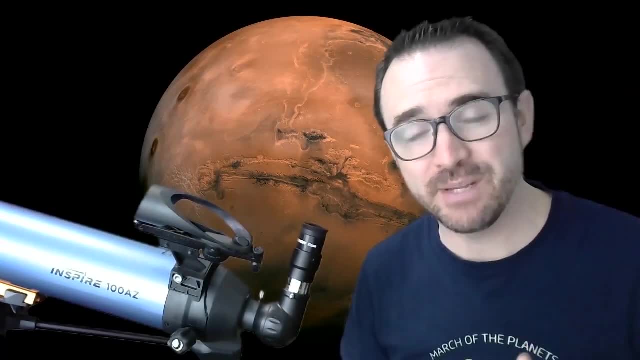 for this technique to work, The third thing you'll want to consider is the camera app that you're using to take the picture. The third thing you'll want to consider are the eyepieces and barlows you'll be using, And this is where you really need to experiment for yourself, Just as it was with visual 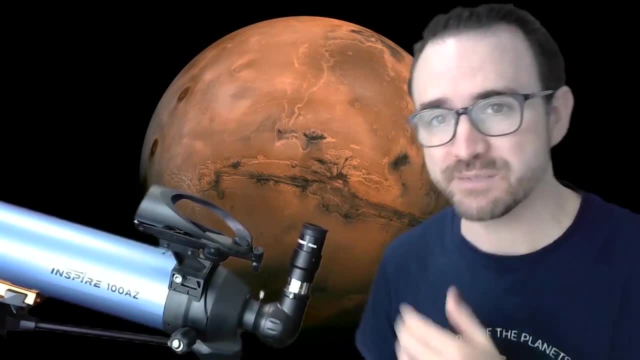 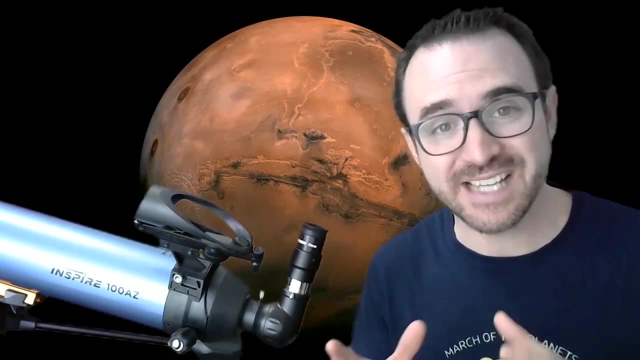 observing, it's easiest to find the planet with the lowest powered eyepiece and no barlow. However, without higher powered eyepieces and maybe a barlow, the planet will appear tiny on the phone screen. So you'll need to find the eyepiece and barlow combination that works best for you. 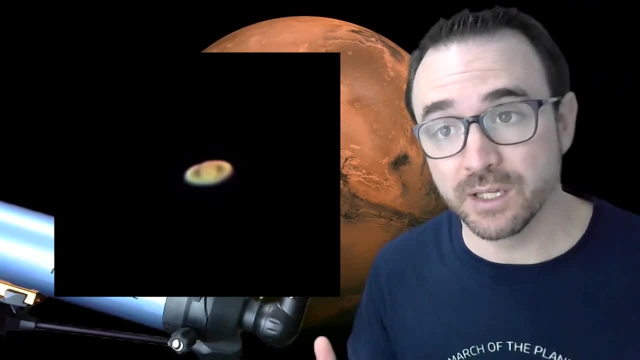 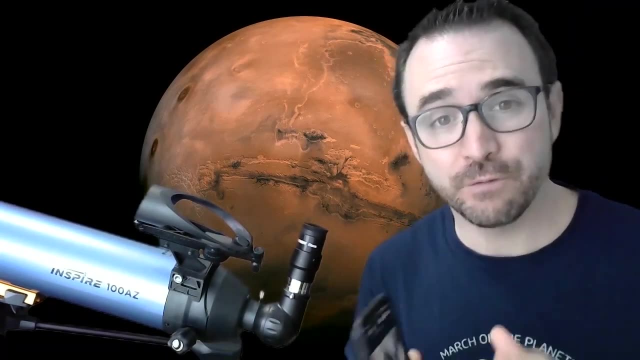 So for this image I used a 20mm eyepiece and a 2x barlow attached to the telescope. So here's how you image the planet. First, you set your phone to video mode. If you try to take a photo using the photo setting, it's unlikely that you'll get a decent image. Next, you want: 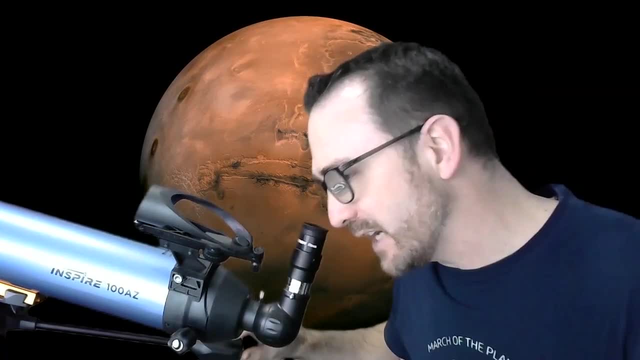 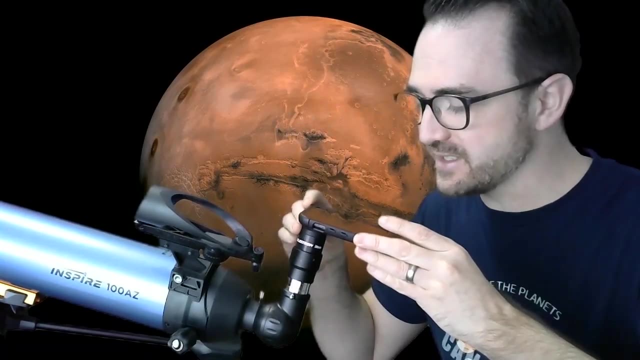 to make sure that the planet is centered in the finder and the eyepiece and that it's in focus. Now here's the tricky part. You now need to get the planet centered precisely on the phone screen and you need to be able to hold it steady. I usually cut my hand around the eyepiece and 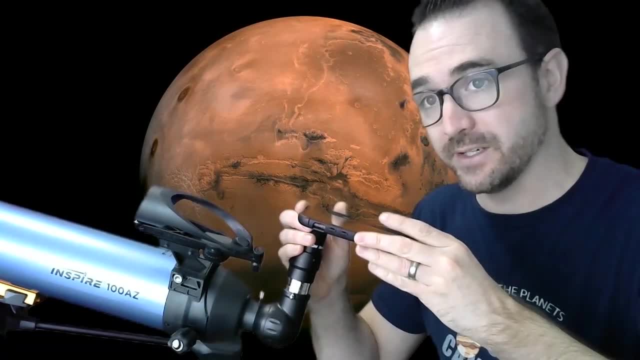 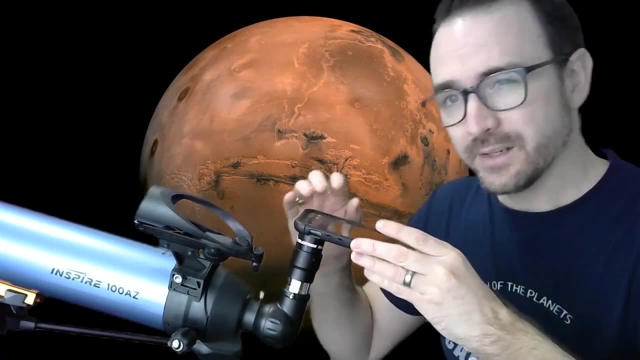 hold the phone, moving it ever so slightly to get that planet centered. Now, it's okay if the planet bounces around on the screen. We're going to fix that when we get this video file onto the computer. Now, once you've got the planet centered on the screen, you're going to want to zoom in. 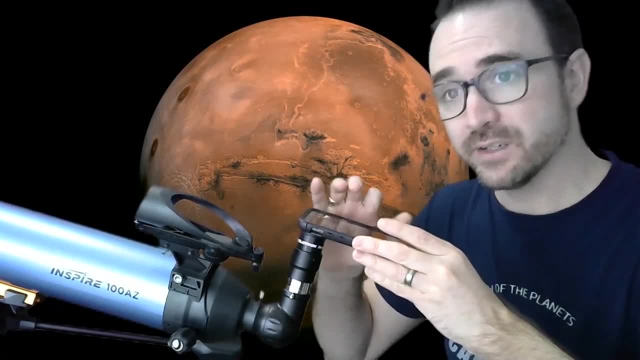 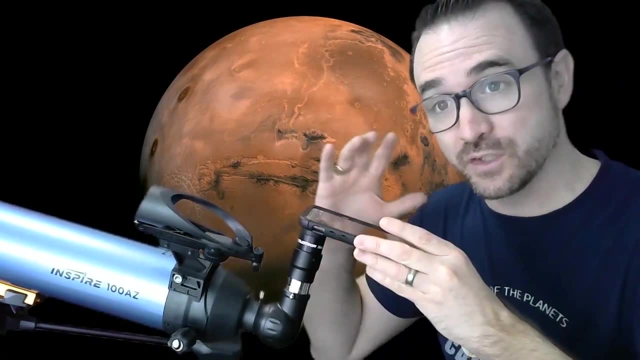 just a little bit. You're going to then adjust the exposure so that you can see details on the planet, as much detail as you can, and you're going to want to make sure that that focus is as good as you can make it. So you'll probably want to do a combination of focusing on the telescope. 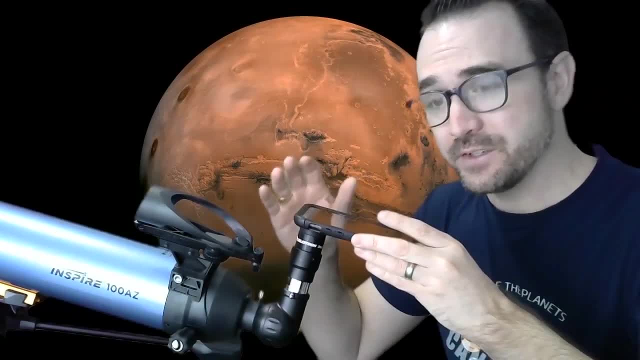 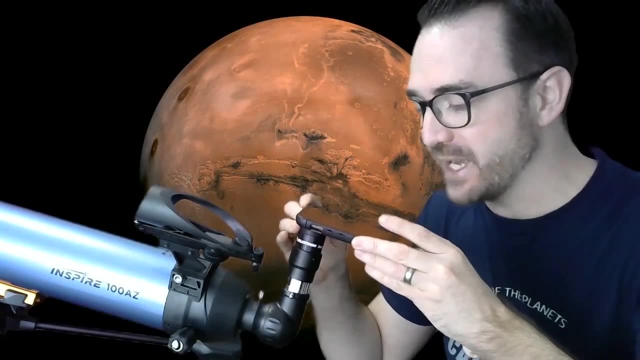 and focusing in the camera's application as well. Now, what you're going to do is take a video Now. the video could be anywhere between 5 and 30 seconds, but for the duration of the video you're going to do your best to see if you can keep that planet centered on the screen. 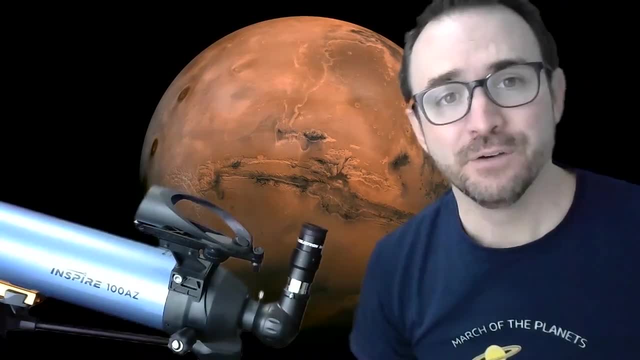 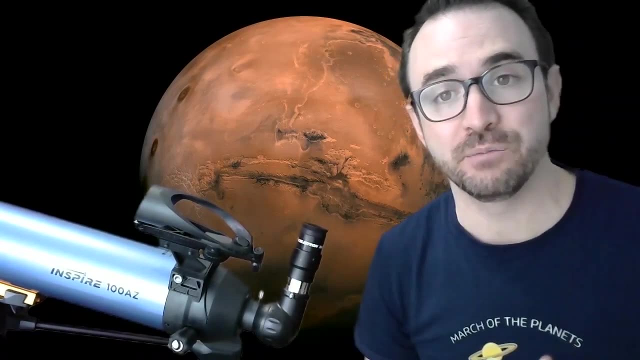 Now, as you can tell, I'm not actually outside, I'm in my office. Fortunately, I did get a video of Saturn using this exact setup about two months ago, So I'm going to move that file onto the computer and we'll pick it up from there. Note that the following process is designed for PC users. 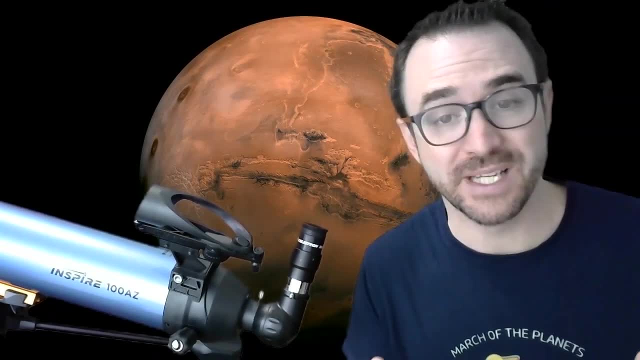 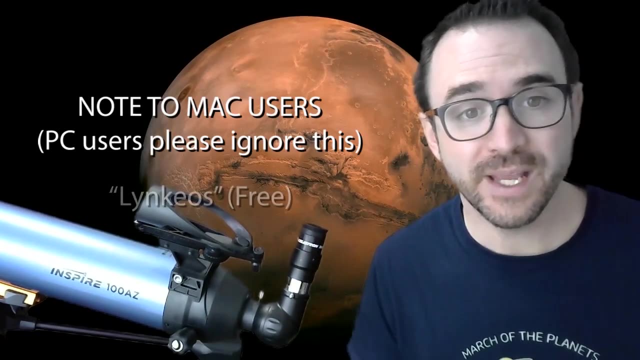 now that's just because most astronomy software is written for PC. If you use a Mac exclusively, there is a similar process using a free piece of software called Linkios. You may need to use video software like iMovie to convert the move file from your phone to the mp4 that this software 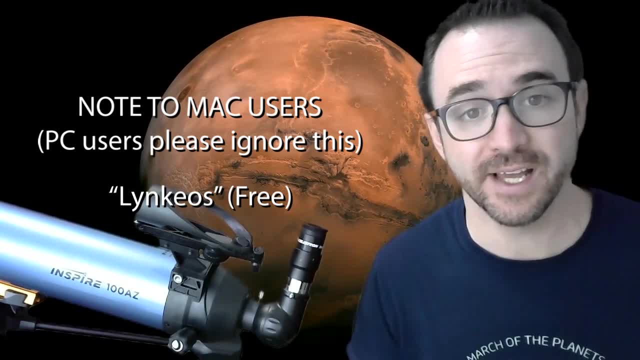 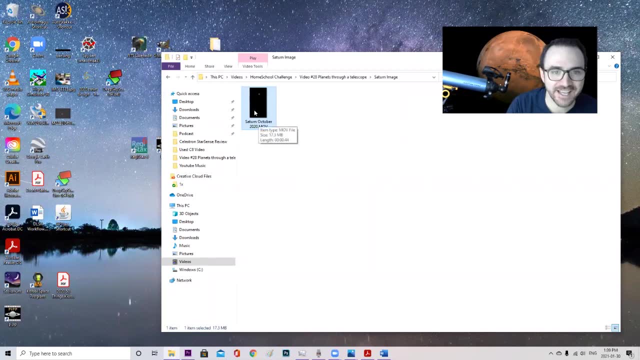 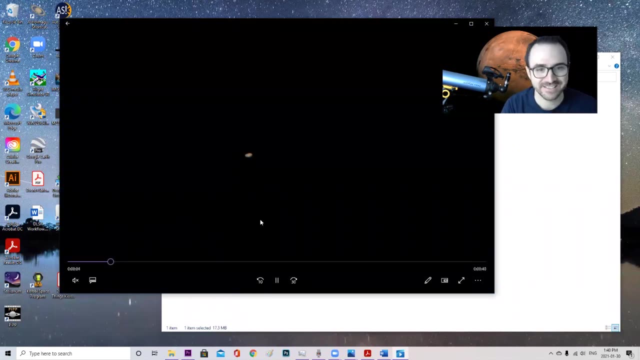 requires. Anyway, there are several YouTube videos on how to use Linkios. I'm going to show you the PC version. All right, so here we are on the PC, and now I've got this video transferred over from the phone to the computer, and so here you can see. here's Saturn. It's. 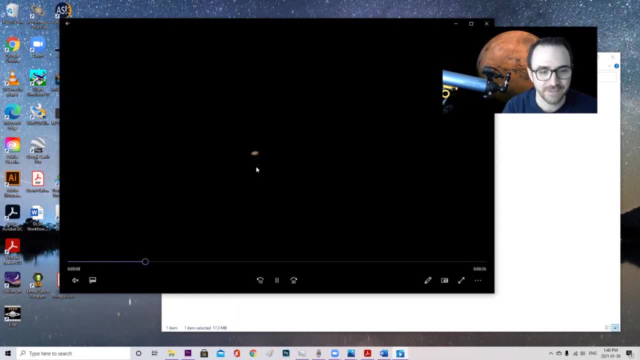 bouncing all over the place and remember, I am just holding the phone up to the telescope's eyepiece here, and so it's wandering all over the place and you can see how big it is on the screen and that's just what's realistic for a telescope of this size. That's about how big it's going to. 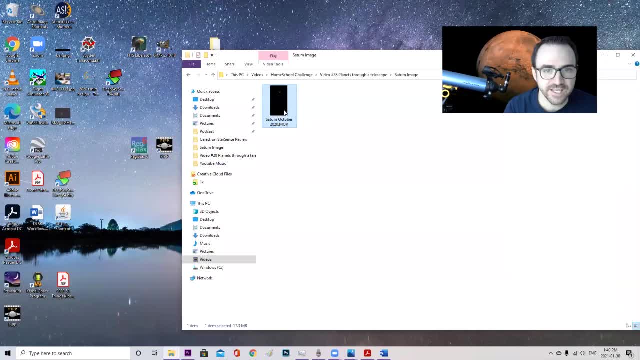 be All right. so I'm going to close this. Taking this video and turning it into a picture that's we can share takes two pieces of software, and they're both free and you can download them off the internet. So the first is called PIPP, So we're going to start with PIPP and the first 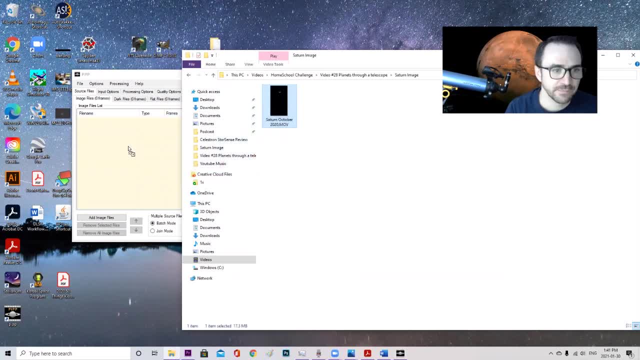 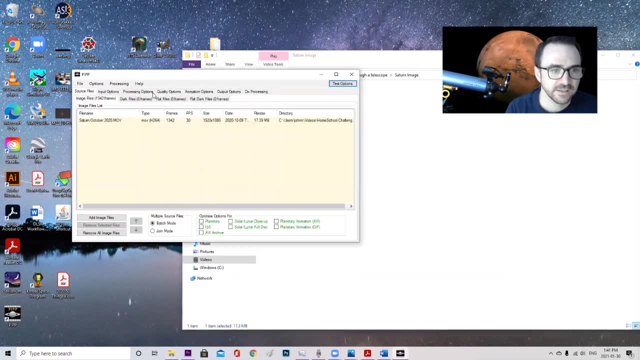 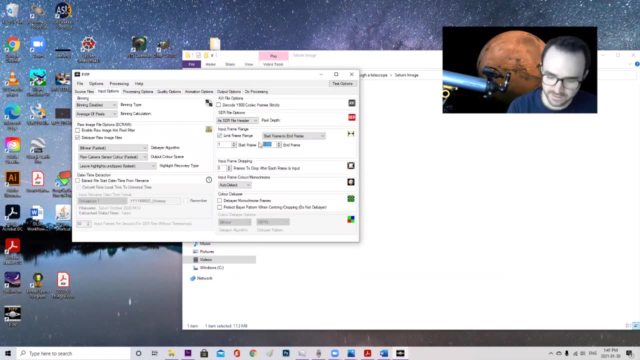 thing we want to do is drag and drop the file from the phone into the software, And here's just a preview of what it looks like. I'm going to close that We can see that this video has 1300 frames. I'm going to take about the first half of those frames just because, in viewing 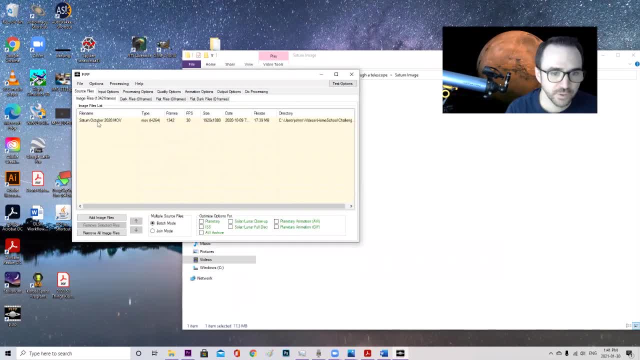 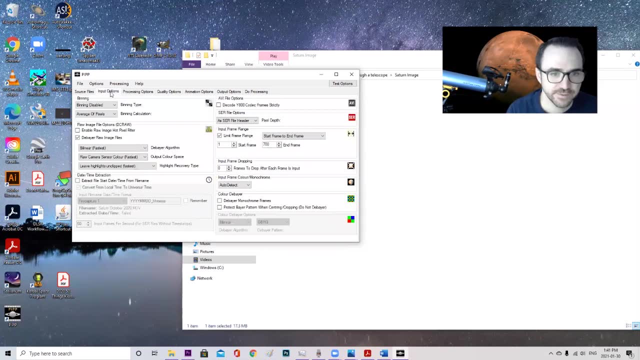 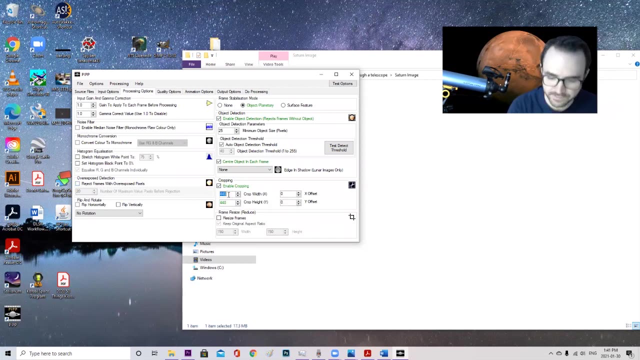 those look like the best frames. Okay, going back to source files, here I'm going to click planetary and that will optimize the file here for planetary imaging. Look at some options here. All right, I'm going to crop this video to a thousand pixels by a thousand pixels. 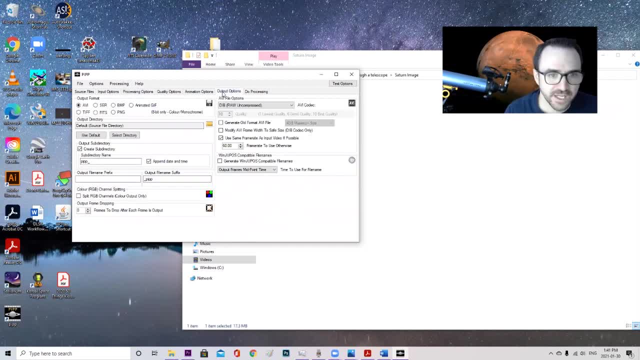 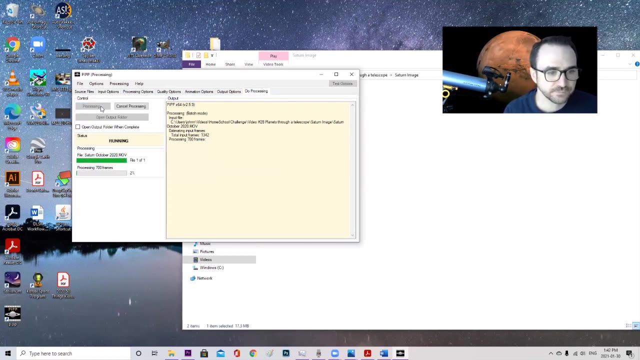 Okay, and then, checking our output options, You want it to be an AVI and to save some space on the computer, I'm going to use a little bit of compression here. Then we're going to click do processing and start processing. What this software does is it's going to take that movie file and convert it into an AVI file. 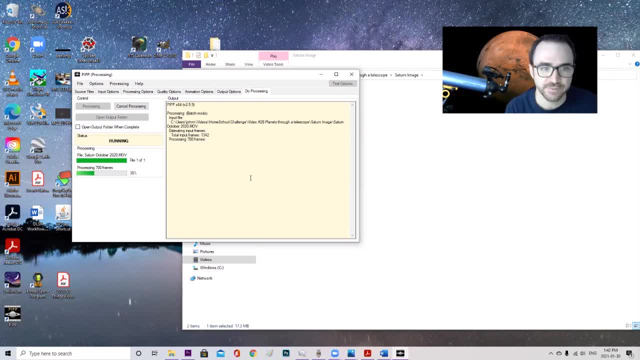 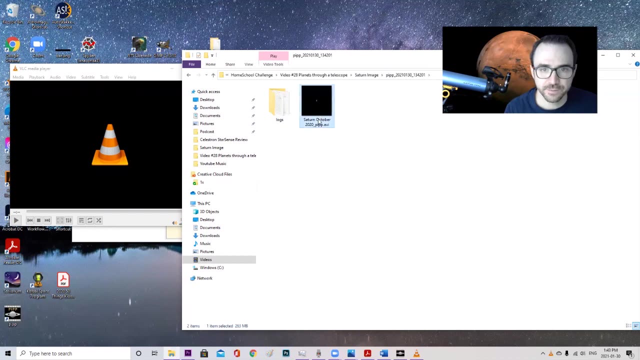 But it's also going to take the image of that planet and center it in the video, and that'll make it a lot easier to work with in the next piece of software which is going to turn the video into a still image. All right, so PIPP created a folder and in that folder we can find our new video file. 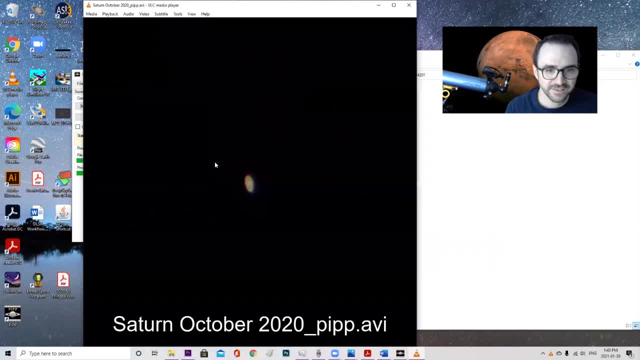 And let's watch that video to see if it worked. There we go. We can see that the video of Saturn is now centered in the frame and now this is an AVI file instead of the move file from the phone. So now we can close PIPP. We're going to open a. 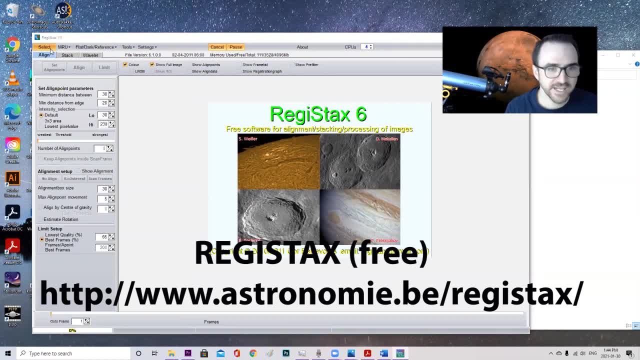 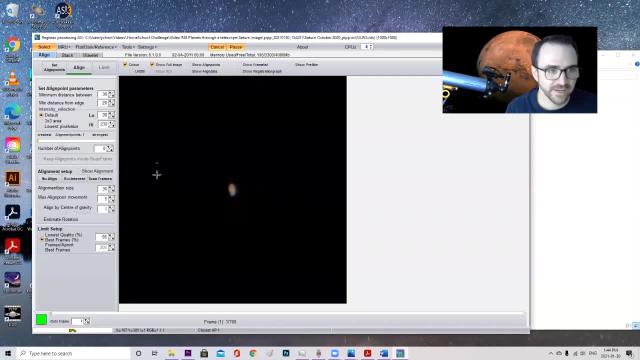 piece of software called Registax. We're going to hit select and find our file. So in the PIPP folder we're going to select the AVI file And the first thing we want to do here is maybe use the slider- This is going through all 700 frames- And pick a good one where you can see a little bit more. 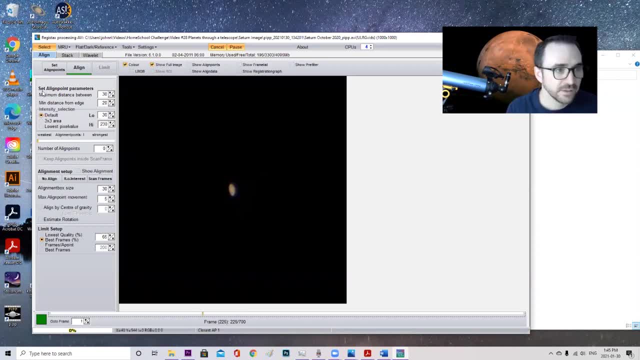 detail than the others. These look all about the same to me. The first thing you're going to do is hit set align points and it's going to choose two. We can add more, and what these are going to do is just tell Registax where the planet is, And then we're going to hit save, And then we're going to 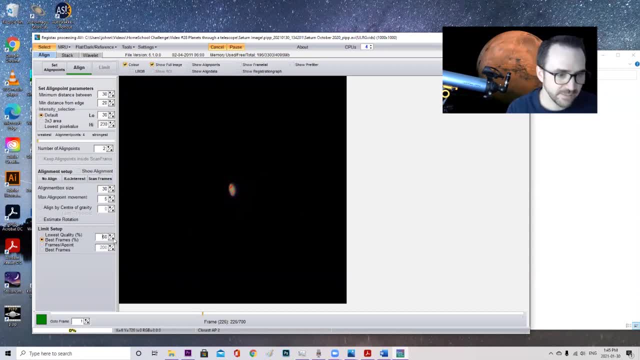 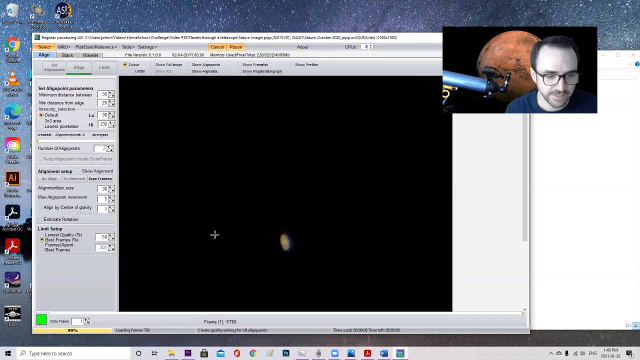 and now all these frames look pretty good. I'm going to select the best, maybe 50 percent, So that'll be 350 frames And we're going to align these frames. So it's going to throw out half the frames and keep half, And it's going to make sure they're all lined up. They're all lined up. 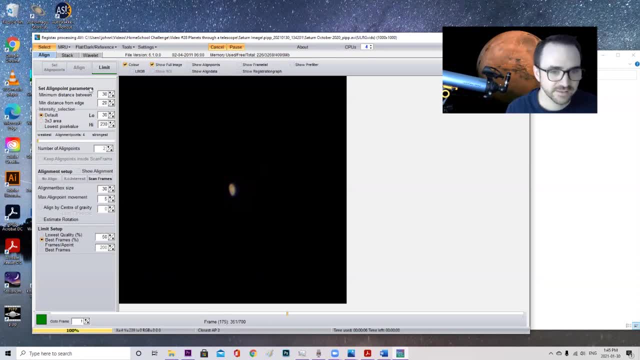 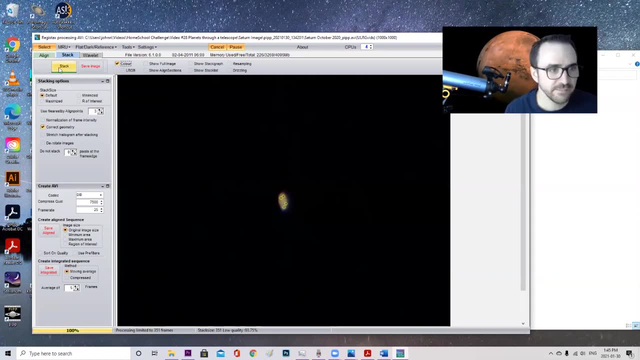 pretty good already, but you know it makes us go through the process. The next thing we're going to do is hit limit And then I'm going to leave all these settings the same And then I'm going to hit stack And this will turn that video into an image And this will take. for me it's